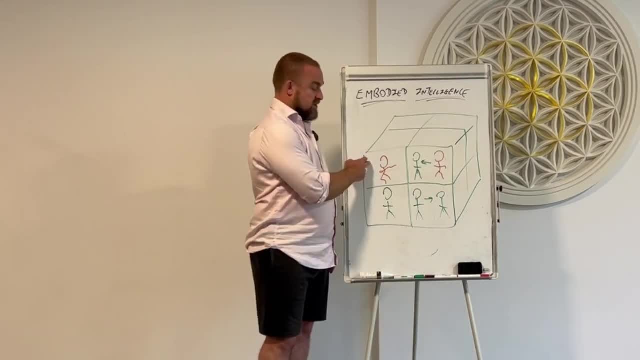 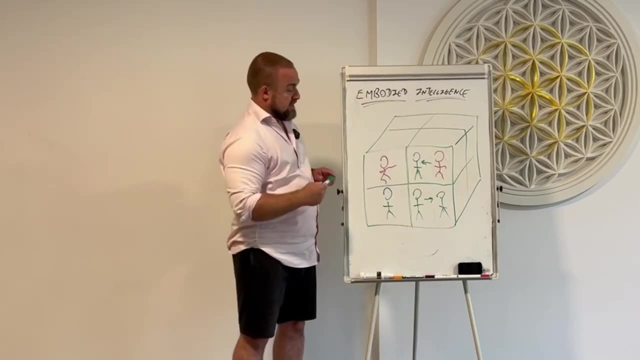 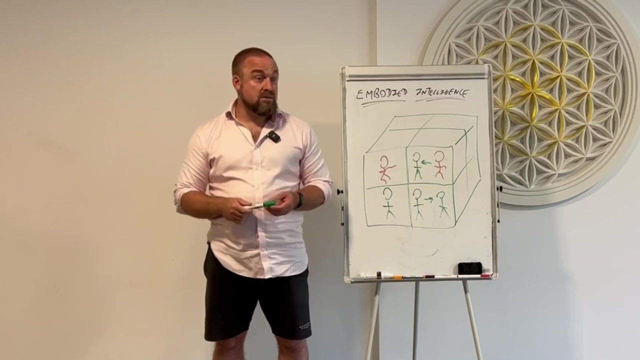 Experientially All right. So first one is self-awareness. Yeah, Self-awareness, So this could be state and trait. So we have two levels here. So we have self-awareness of our state. So when I say what's your energy level like today, Or I say, how are you Right, This is what we're. 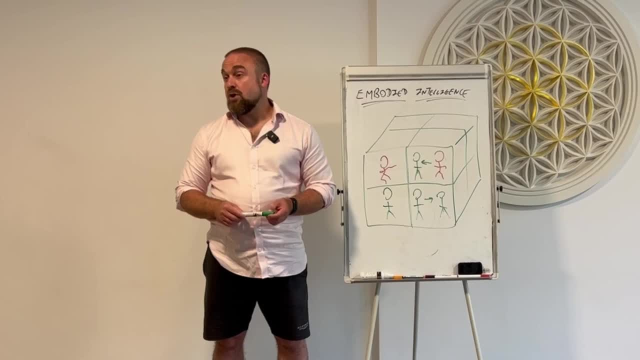 asking: What's your state? So, as a facilitator, that's really important. I know that. So if I come in, I'm in a bad mood. I need to know. I'm in a bad mood, Yeah, Or else I'm going to teach. 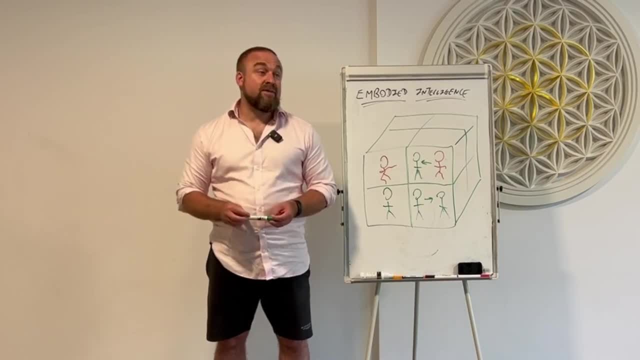 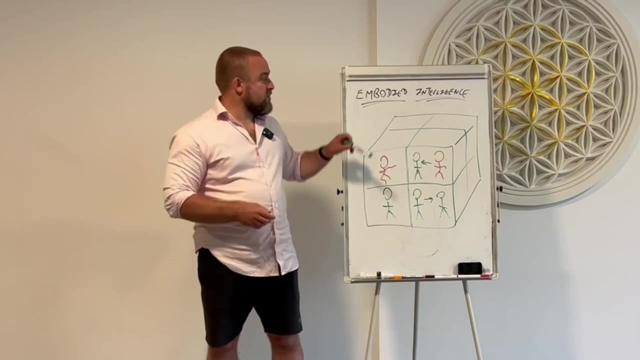 very differently. I can Factor that in or usually factor it out. So I need to know my state. Okay, If I'm very tired, I need to know that. So that state. we've also been working with traits here, Okay. So this is we can. 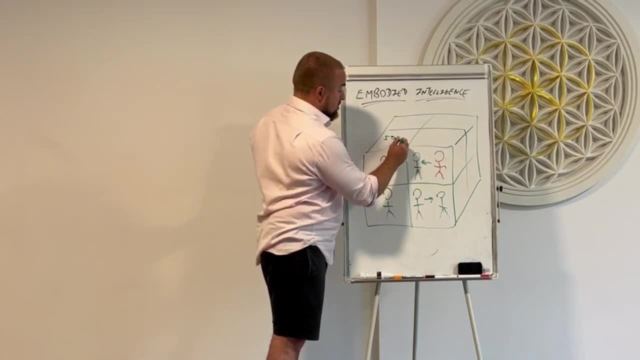 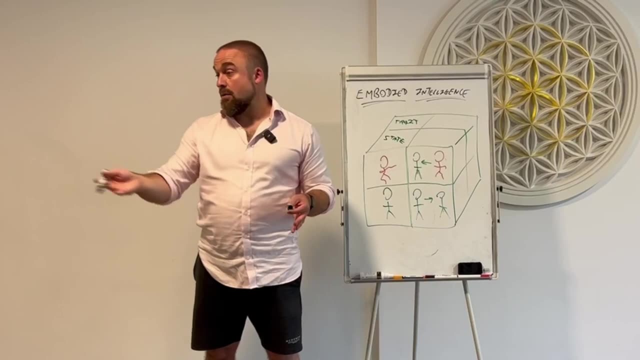 say it's like short-term and long-term State's actually the easy one, because you can just feel it. If I say to you, how are you? You're not a child- You can tell me, Like Renko, how are you? 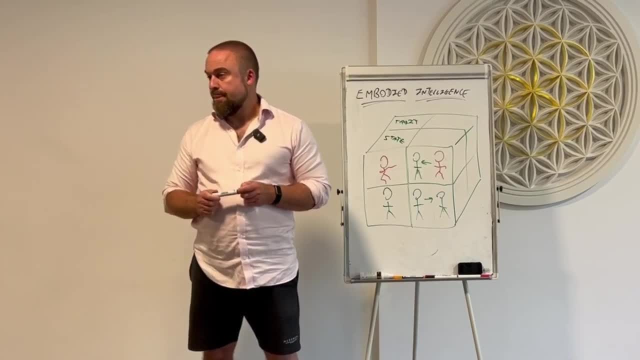 Quite fine, Quite fine. Give me a better word for it And Jeff can tell you: Good level, not tired, Not tired. Good emotion, Reason to be happy, Yeah Yeah. So like still takes a little bit of noticing, right, Because normally we say I'm fine, I'm good. 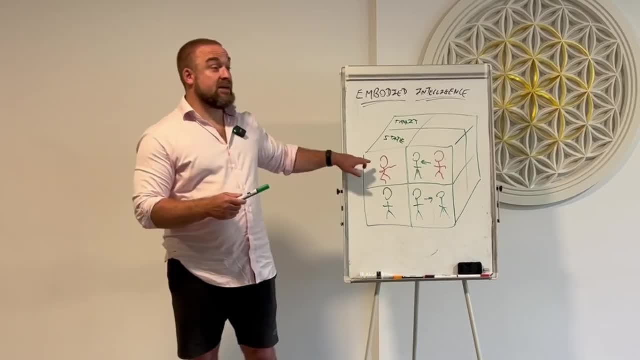 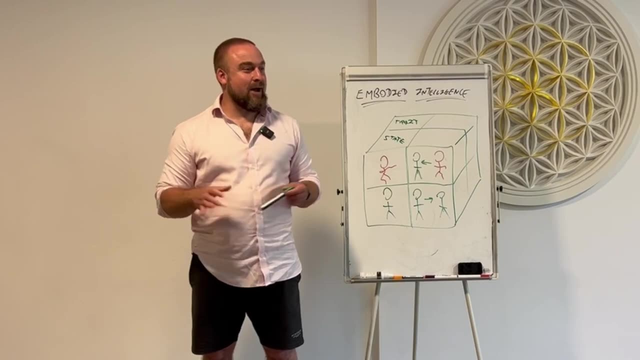 And then it's like: nah, actually we can be more accurate, So you can still build skill in this level. So Dimitri's an MVC trainer, for example. like people often start out with not much skill, You know they go, I'm fine, I'm okay. I often say to my students: okay, find a band, just getting. 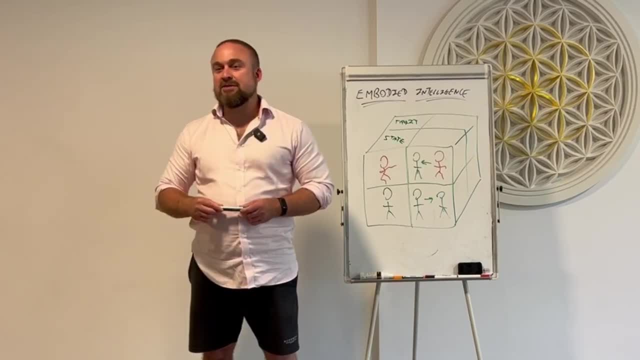 people to name it, And then we practice on our courses. you know, five times a day You have an alarm that goes off and you go: how am I really? That's a skill. Okay, You can get better or worse than that. I gave the example of a child. He's like: I'm not tired, They're worse. 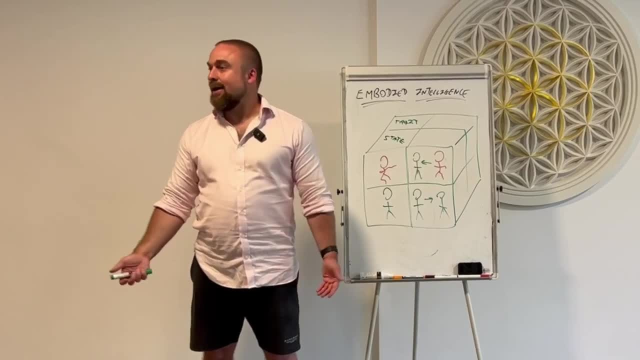 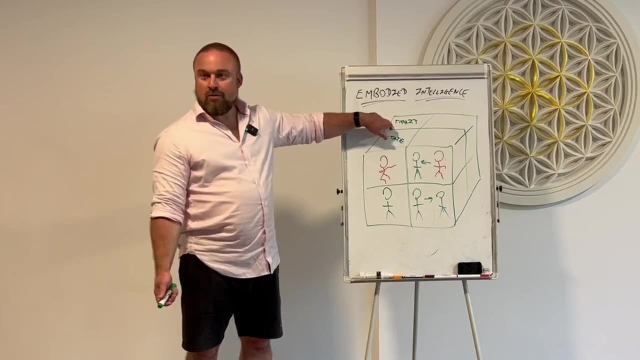 at it. Okay, As they get older, they get better at realizing: okay, I'm tired. Yeah, All right, Trait, you cannot feel It's the taste of your own mouth, Or an example one of my colleagues gave- is the smell of your own house. The only time you smell your own house, When is it? When can? 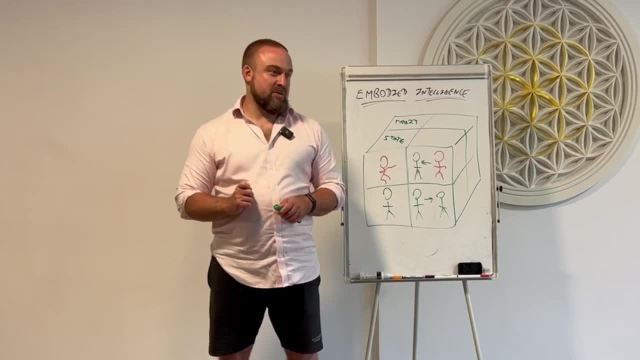 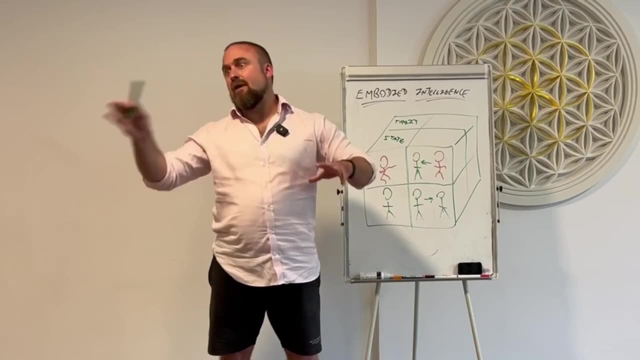 you smell your house When you come home from a holiday or a trip? Okay, Because then you're unhabituated to it. Yeah, So one of the things we can do in life is one we can just change environments. that can maybe reveal something. You know, you go to the 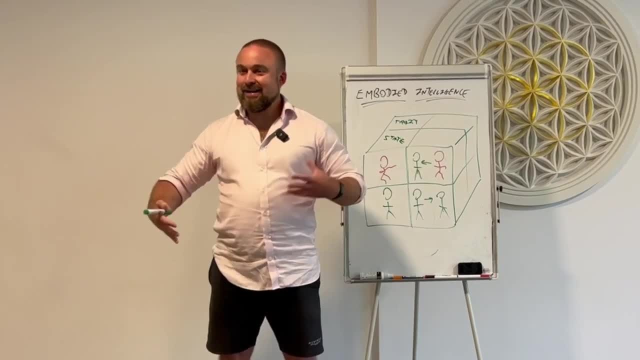 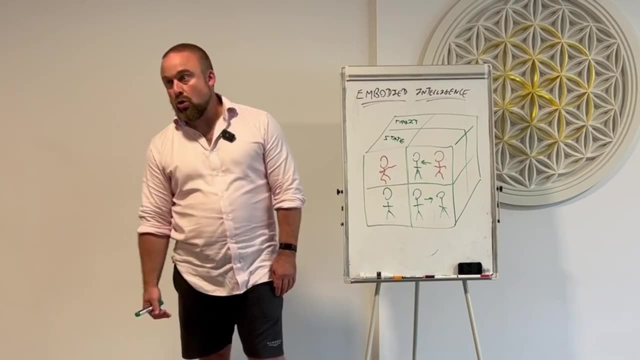 Mediterranean, and then you're like, oh shit, I'm in another culture. Ah, I feel different. Yeah, So this has aspects that are more personality, that are more cultural. They're all mixed in together. The difference is they're more longer term, And the other way you notice is the techniques. 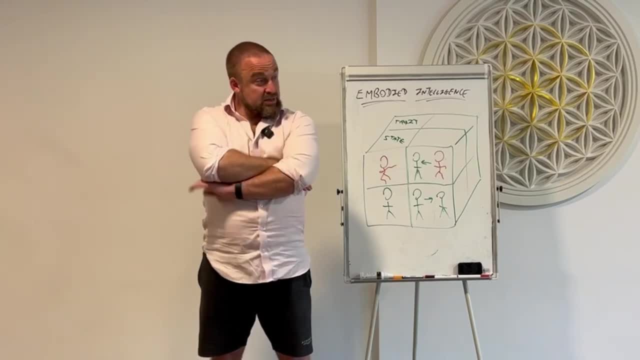 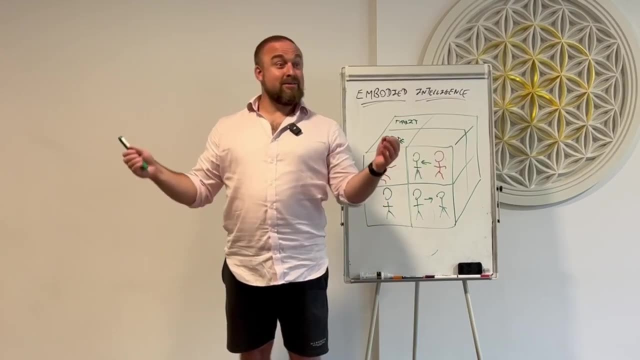 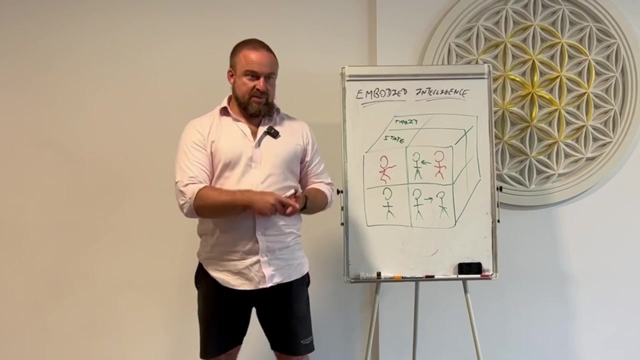 we've been using today. So one way is you try two things, You try this and then you try this. Or we did like Gary And then we did what was the spiritual lady called Shanti. We did Shanti and we did Gary. Okay, And you do both and you go: ah, which feels familiar. Okay, So what is? 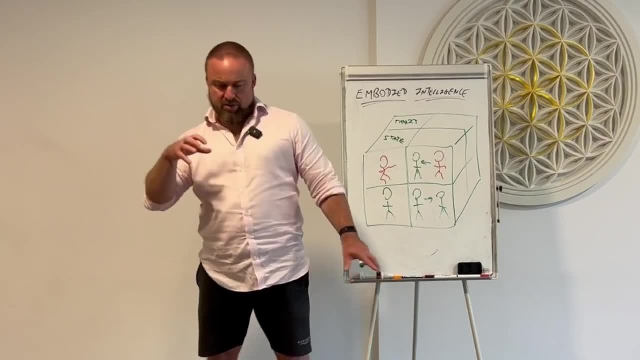 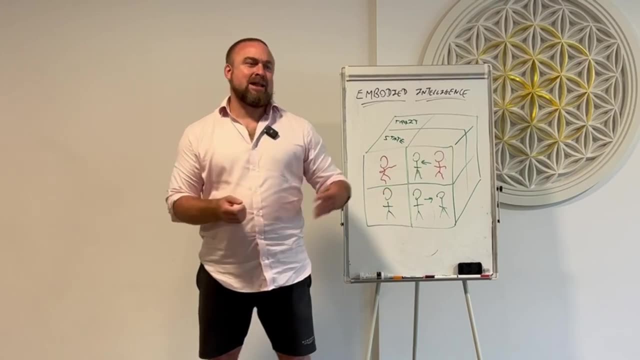 familiarity. The other one is kind of taking you out of an environment. Third one is feedback. So we said two people would tell you today what are you not? And we're doing this playfully- What animal are you not? Whatever, Two people say you're not a shark. Okay, There's some trait of sharkiness. 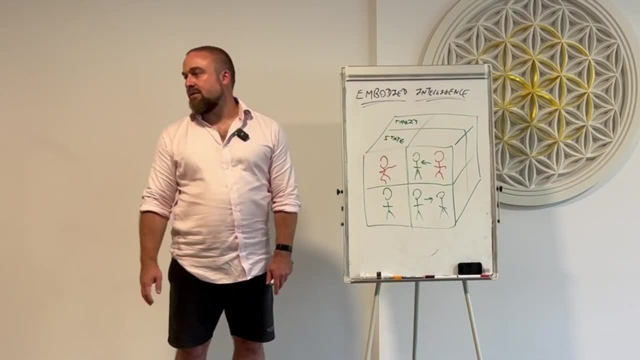 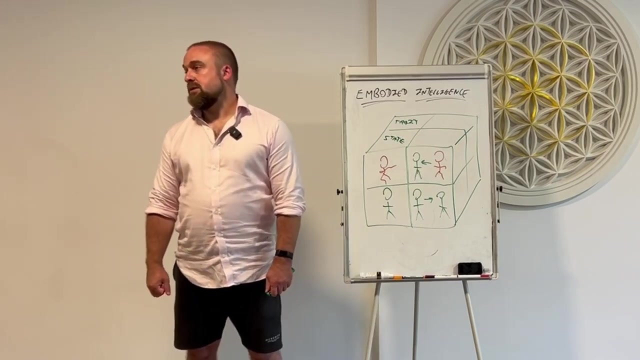 It might be like, you know, direct, aggressive, predatory, whatever that you're getting feedback like: ah, okay, Maybe I don't embody that so much Exactly, Yes, Yes, Yeah. Or the third one is something like putting yourself in a very novel environment where it's exposed somehow. So we have. 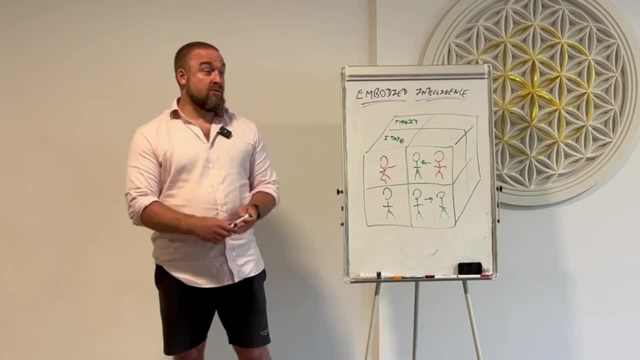 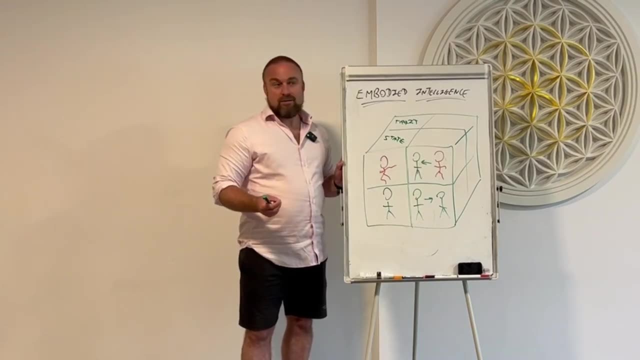 to expose trait. You can't feel it. So, mindfulness: you're in a yoga center, right? It's only good for trait. You can meditate as long as you want. You're not feeling your trait. You're not feeling your. 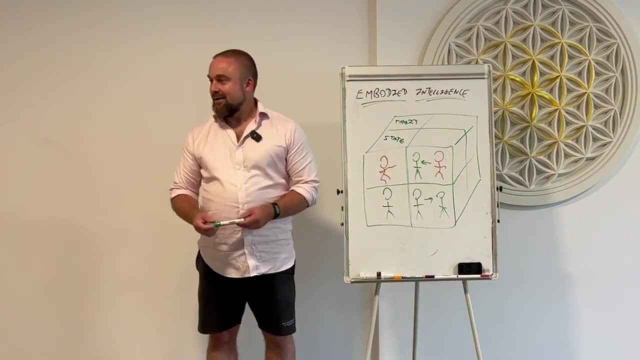 personality. It's like, oh, I'm meditating on my extrovert. Yeah, I mean, it will still get revealed if you do a meditation retreat in some way, but it's not. you're not mindful of it, Okay, So 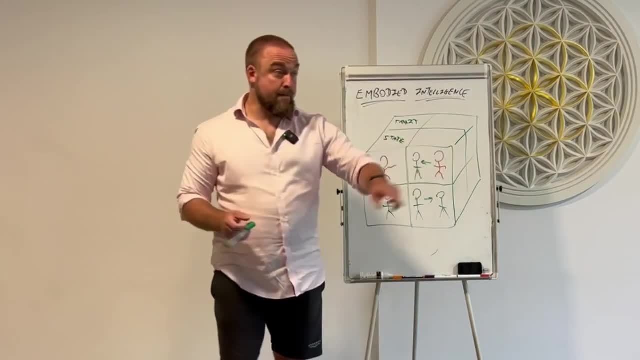 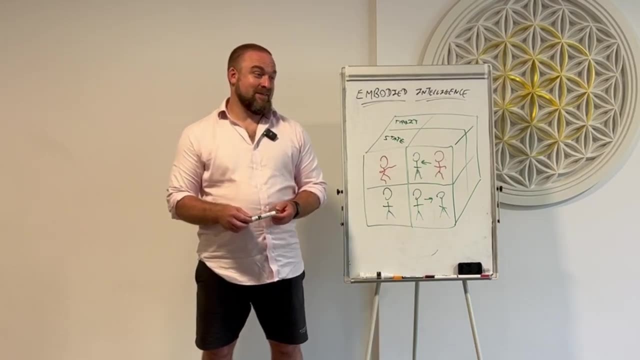 mindfulness is great for state, not for trait. Yeah, Yeah, Yeah, You could. we could have done it that way. One is just playful, I'm having fun with it. The other one is we're looking at like what's not allowed, So what we've got in state. if you. 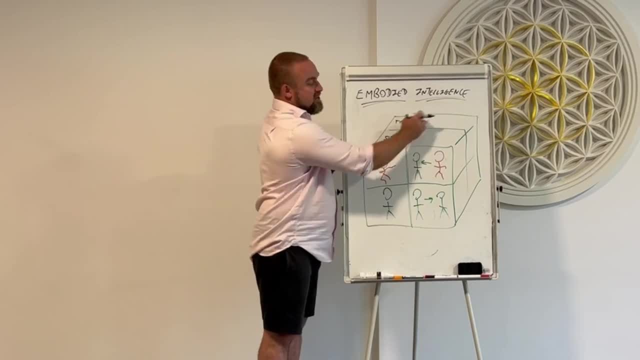 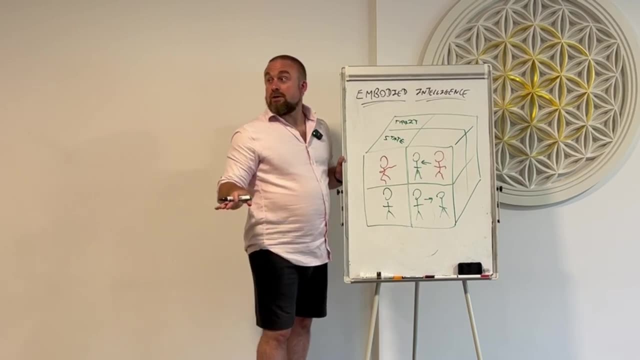 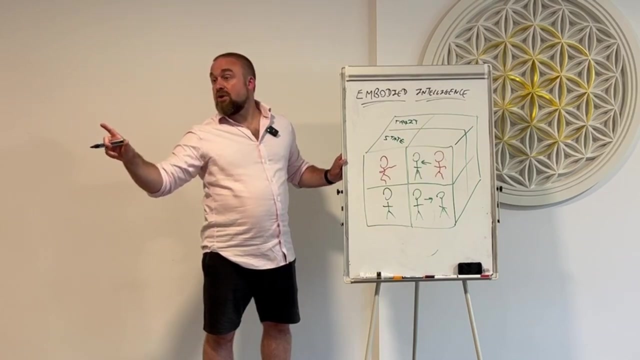 imagine, okay, imagine. this is all this square is all the human possibilities. And when you're young, children have a lot of possibilities. When you're young, you have a lot of possibilities. What's the word Trait? We need a translation Slovenian for trait. 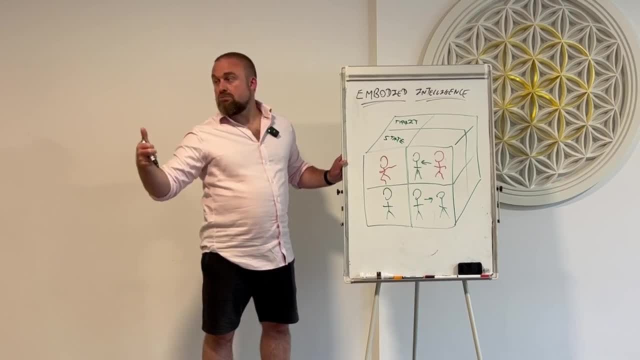 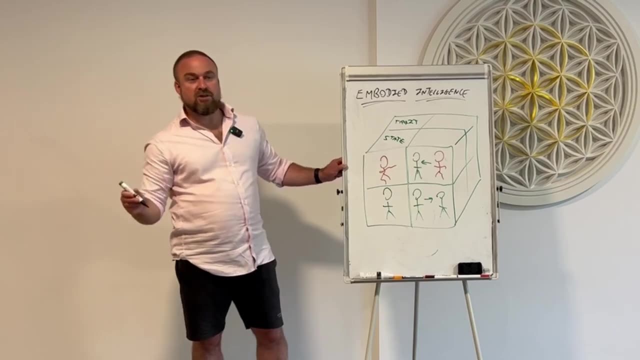 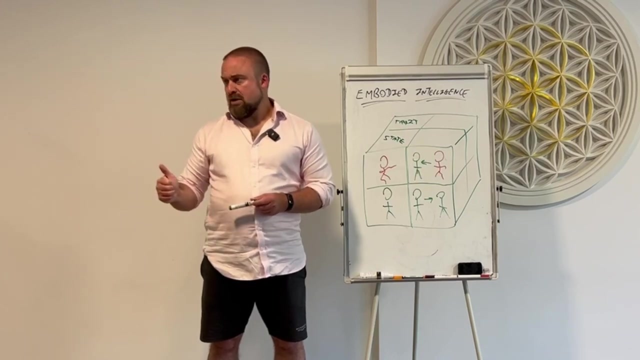 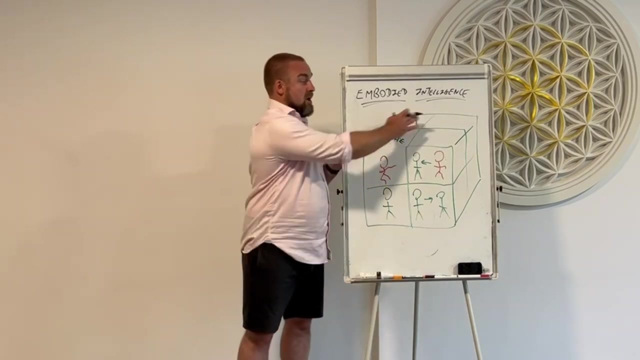 Yeah, Is it clear? So it's a longer term characteristic of your, you know, personality, character, you know something that doesn't just immediately change. It's clear, clear enough, Okay, Where was I? Yes, So what are you not? So if we imagine that when you're young, you have all, 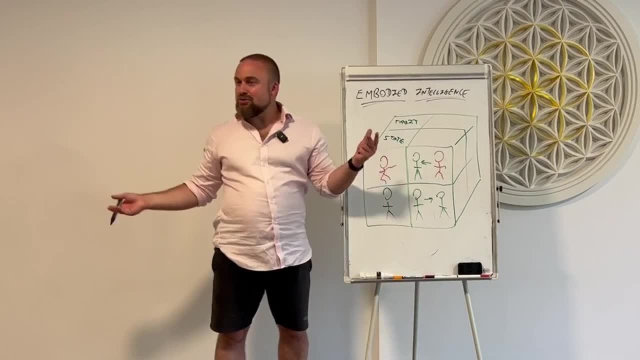 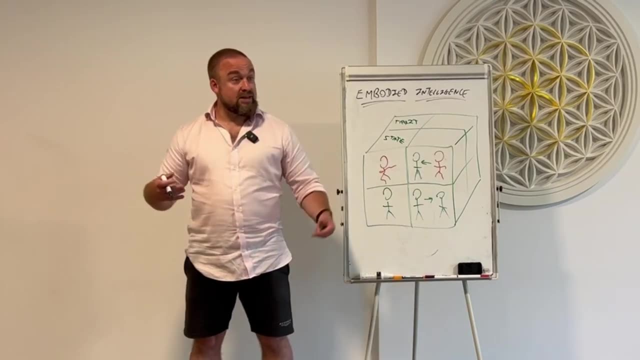 these possibilities right, And you see a child, they'll change their emotions. I love you mom. I hate you mom. You know they're really like changing quick, Yeah. And their posture is also not condensed, It's very relaxed, very soft, very aligned. They're not like tightening into a 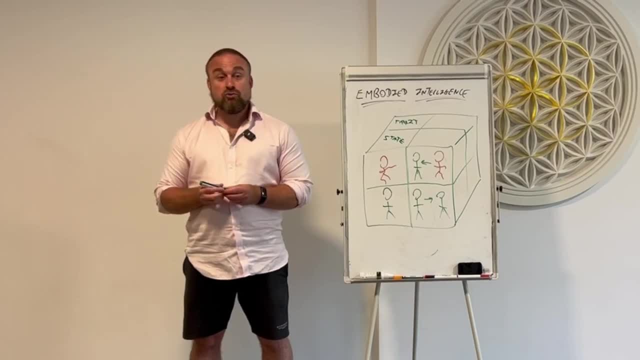 particular posture. If you look cross-culturally, children are more similar cross-culturally Adults, you can see they're enculturated. Yeah, You see, like a little Polish kid. They're like, hey, you see like a Polish man. Yeah, You see a little Japanese kid. Oh, same as a little Polish. 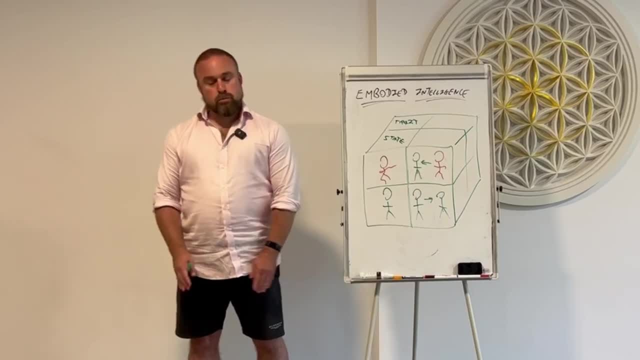 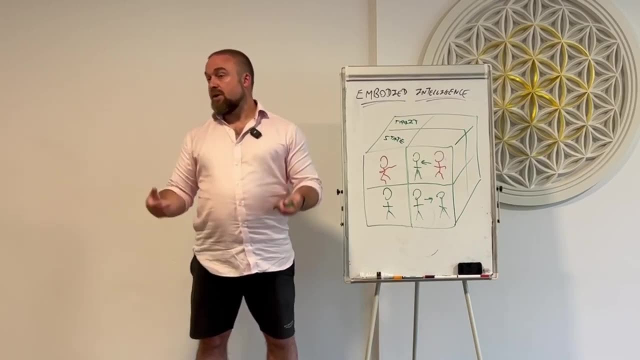 kid. Just you know it looks different, but same posture, same everything And, after a while, more Japanese. Yeah, Because the culture forms the body, Same as the personality forms the body. It's always this combination of personality and culture, Yeah, Okay, So you can think of it like: 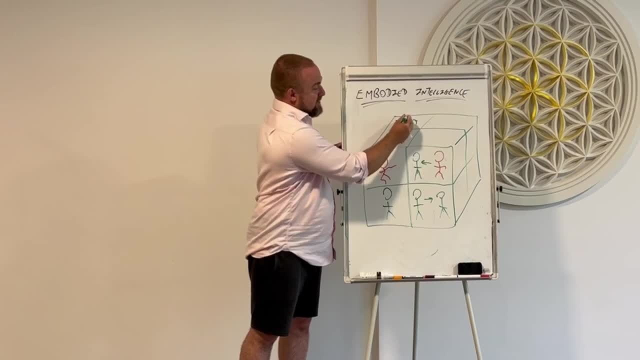 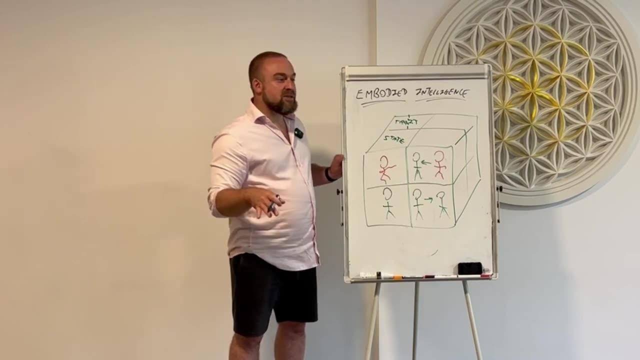 what are you not? There's almost two levels of this. If we take a trait like this, All right, What are you allowed? This is everything that you're practiced, in that you're good at how you want people to see you, what gets you what you want. We did this exercise. 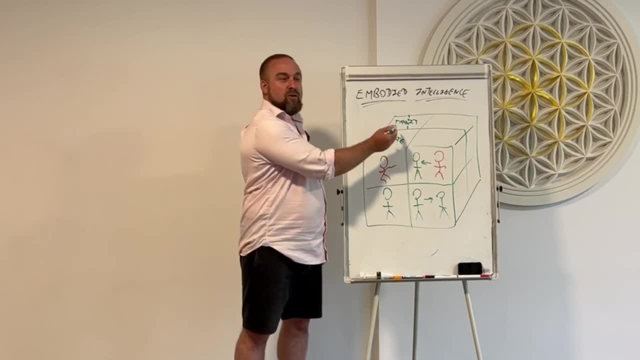 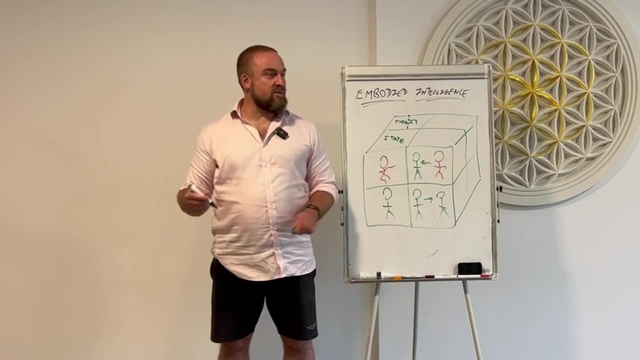 make someone like you. You immediately went to your traits that you're already good at And you had some skill, like some of you were charming, some of you were helpful, some of you were clever, some of you were funny, some of you were sexy. These are all traits, right They're? 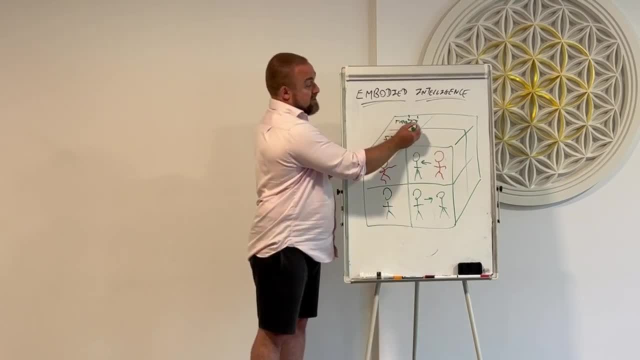 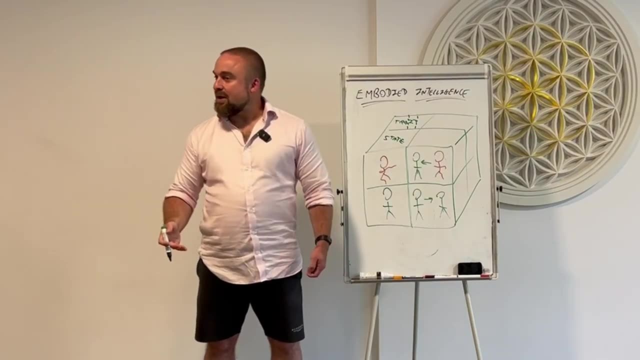 characteristics. There's other stuff that you're just not very good at. Yeah, So some things like: ah, I'm not a shark or I'm not direct. Okay, I'm not, whatever, it is Right, We're just playing games with this. There's other stuff, though, here that you're not allowed to be. That's the stuff. 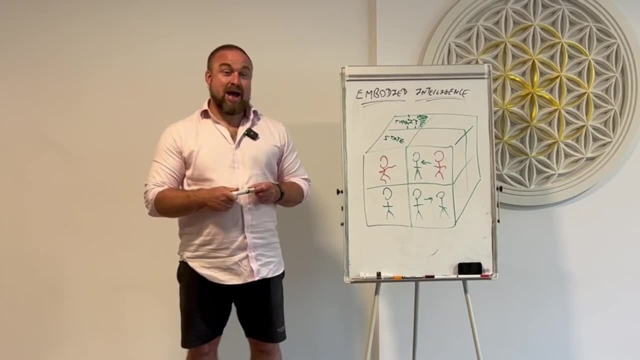 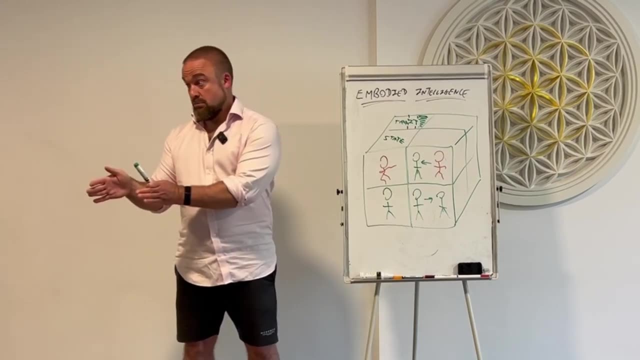 that's like: actively dangerous. Okay, So your pattern, your trait, has said: you can be this, You could be this, but we don't do it very much, but you're not allowed to be this. Does that make sense? So they're like: what are you not? 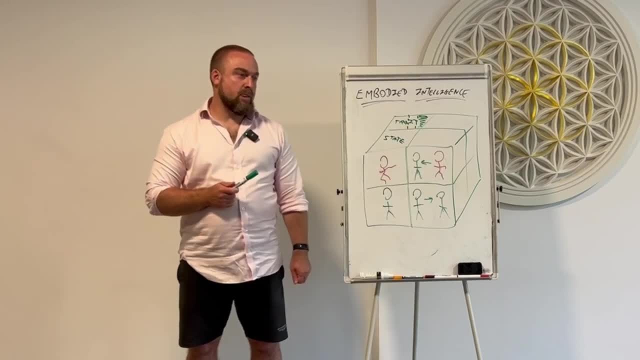 In some ways, we're exploring this other side a bit more. Yeah, But we could have explored what are you Good? So we're learning to extend our range, awareness and choice. That's the basic thing. We've become aware of the emotions, the states, the moods, and we can change that. 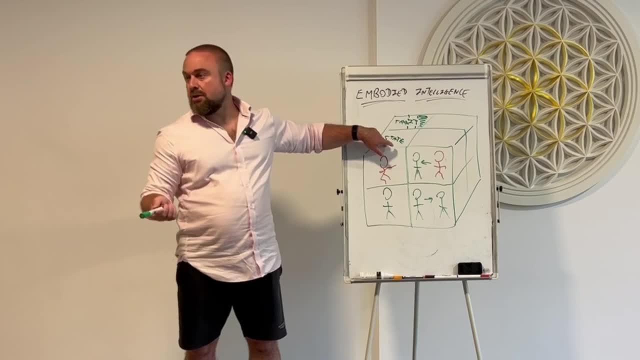 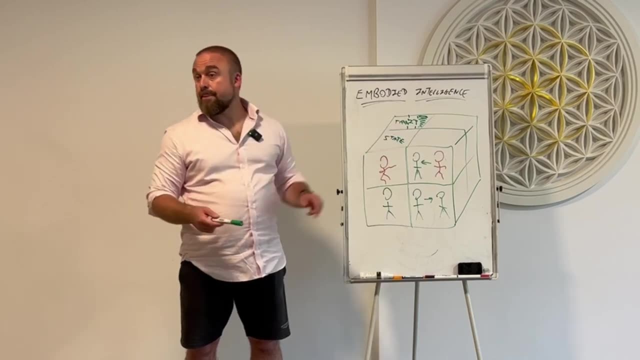 I reduced my anxiety while having the medical procedure. It changed my states. How do we change traits? There's really only two ways. One is practice, The other one is immersion. Okay, So, if you go do Kung Fu for 10 years like Anya, uh, which immersion being like. 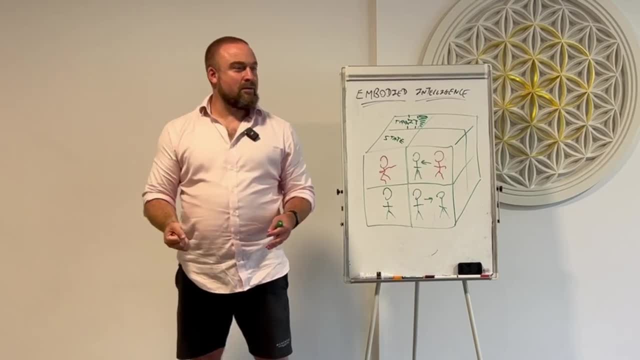 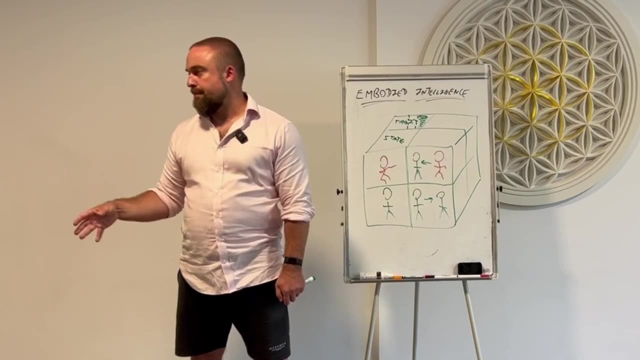 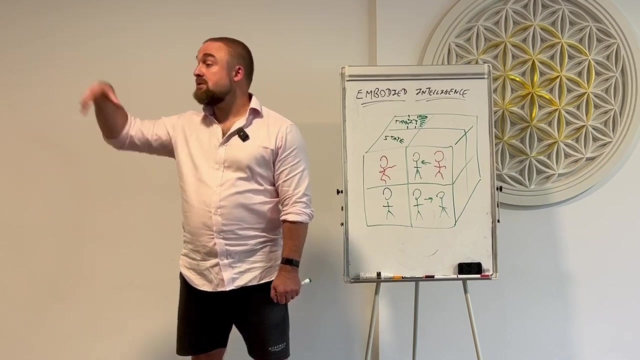 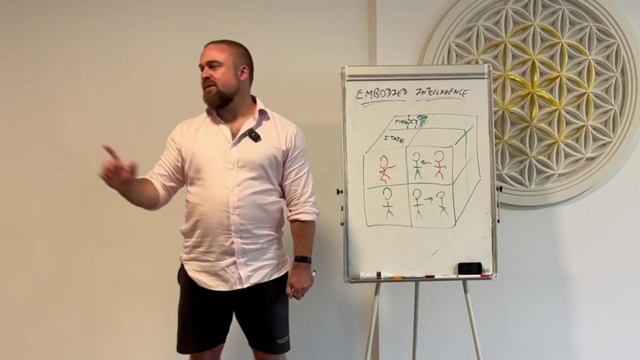 put in the water. immersion, like, uh like. if I go live in Slovenia, that's immersion, being placed in an environment of. so it makes sense. So if you go live in Japan, you're immersed in Japanese culture. Thank you for asking. Good, Yeah, But it's a language thing. Do interrupt me. 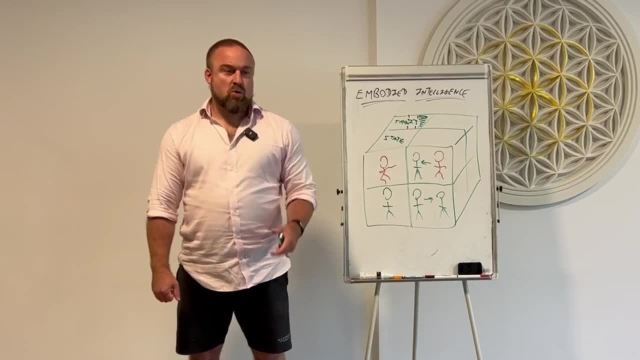 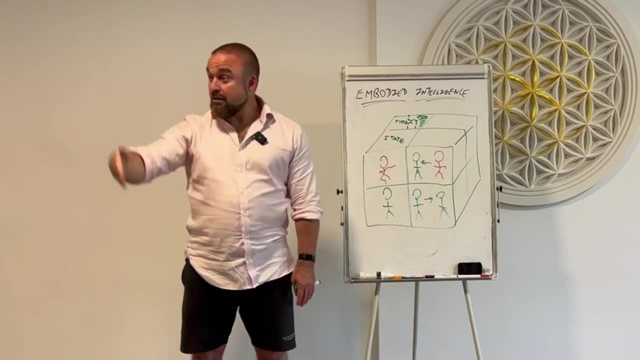 because I want you to understand: Yeah, Good, Yeah. So what is practice If you go do Kung Fu? how long have you done Kung Fu? 15 years, Okay, And you can see it in her. You see the Kung Fu. 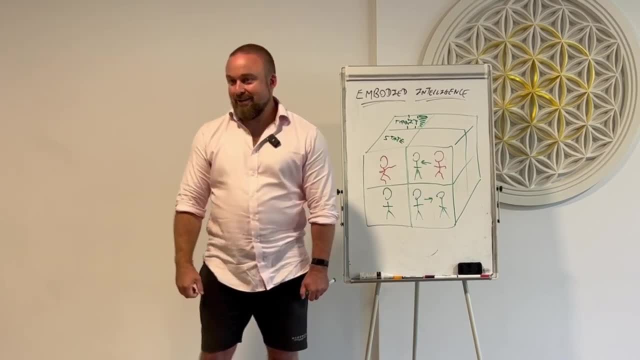 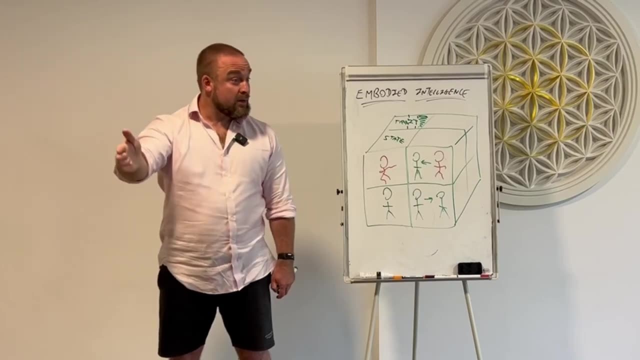 in her. Look how she's sitting. She's sitting like a bad-ass Shaolin monk. Okay, She's not slouching on the wall, She's sitting. you can't see this on camera. She's sitting like a fucking Shaolin monk. right, It's in her body. She doesn't have to think about it. She doesn't have to think about it. 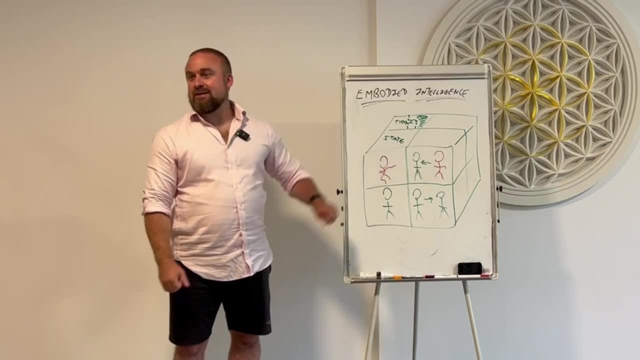 anymore You have to think about it. when it's state, When it's trait, it's a default. That's good and it's bad. Why is it good? Because you don't have to think about it. Why is it bad? Well, because it's what you do without thinking. You with me. 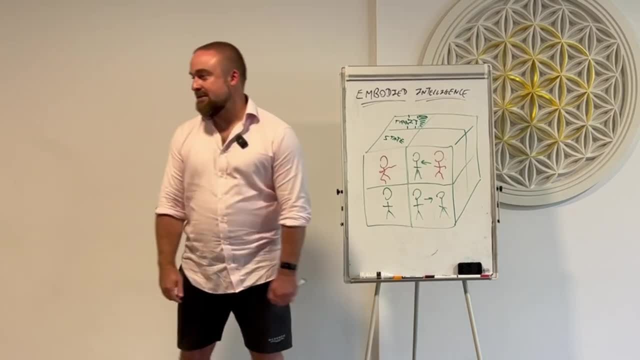 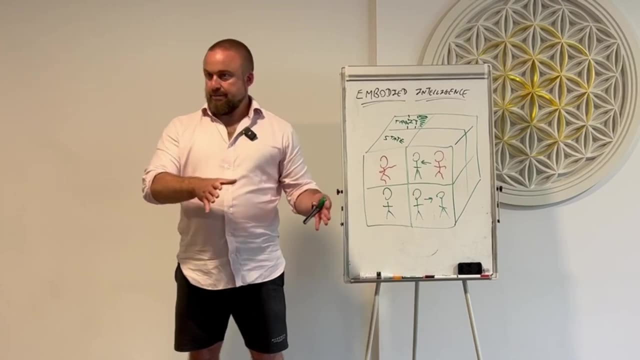 So it's a default. She sits like a Shaolin monk. You can see that in her. Yeah, It's not bad. Okay, It's a positive thing, but it's also a habit. Yeah, Traits are habits. Okay, So it's good that the habit is bad. 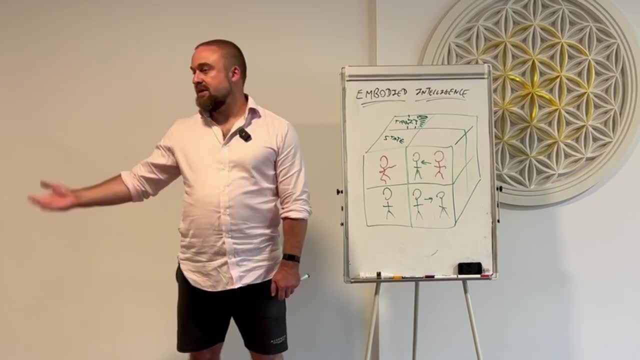 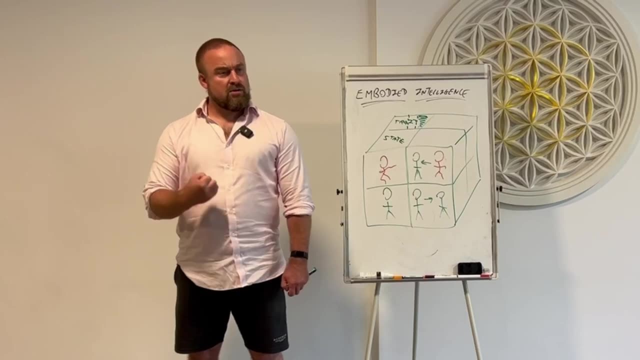 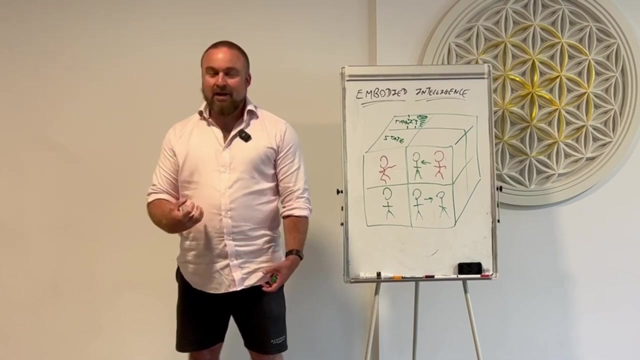 All right. So one way is practice. You go do something for 10 years Like I used to work, used to work in Russia a lot And most people in Russia are like quite severe. They're not very happy, They're quite like, they're quite strong, but they're a bit severe. And I had one friend: 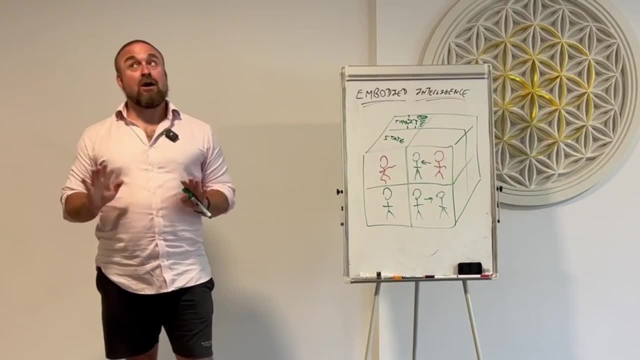 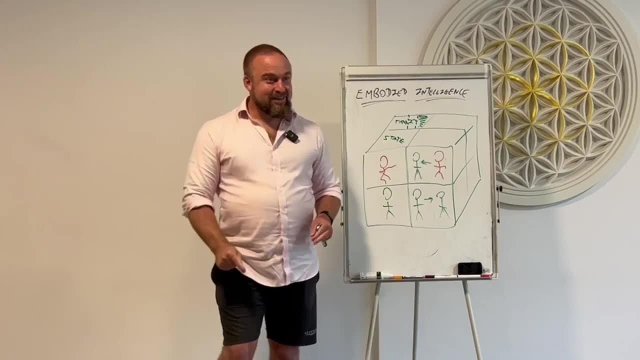 who was like this: Yeah, This girl I used to date She was. I used to love dating her in Russia because she was so much fun and everyone else used to depress me a bit, But she'd be like she was a salsa teacher. Yeah. 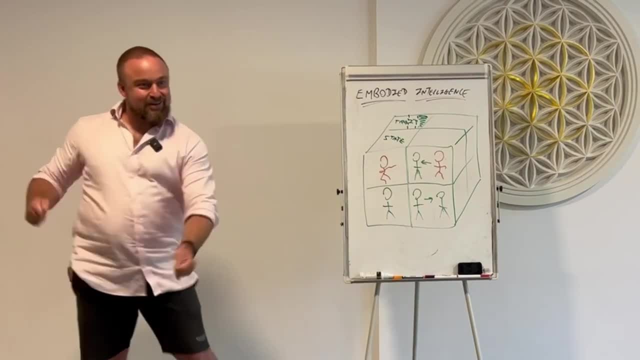 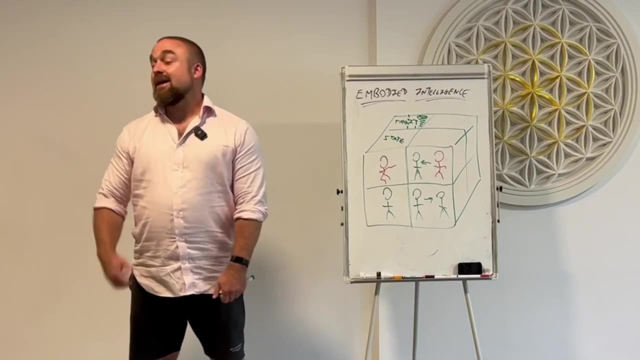 She's like, Hey, come here, It's nice to see you, Mark. You know, she was like happy dancing. She had the energy which for me was like, Oh, thank God, When you're in Moscow in the winter, Yeah, So that again, that was a practice for her, Different practice than 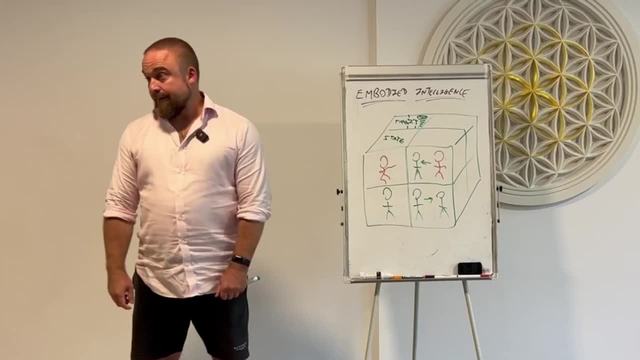 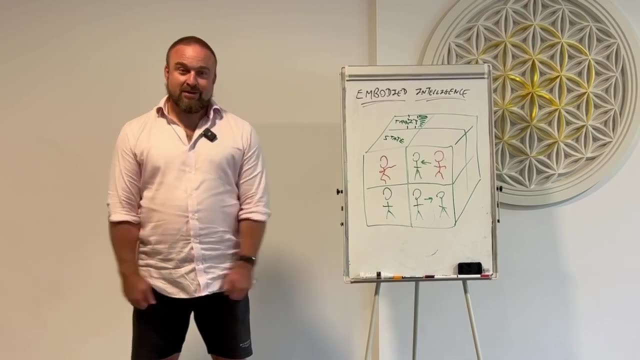 Kung Fu, Different energy, different embodiment energy, Right. Yeah. The other way is just immersion. You go live in Japan for 20 years, You'll change. Okay, If I move to Slovenia, stay here for 20 years, I'll start getting Slovenian. Yeah, At least to some extent. 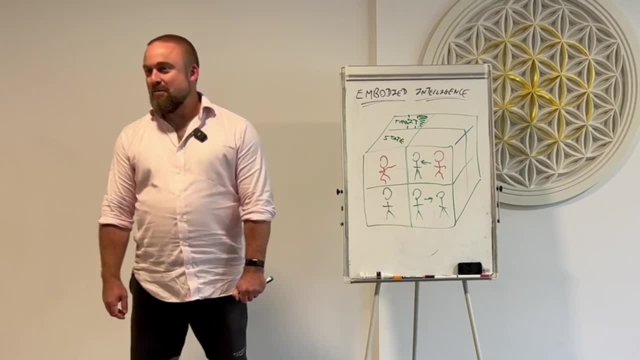 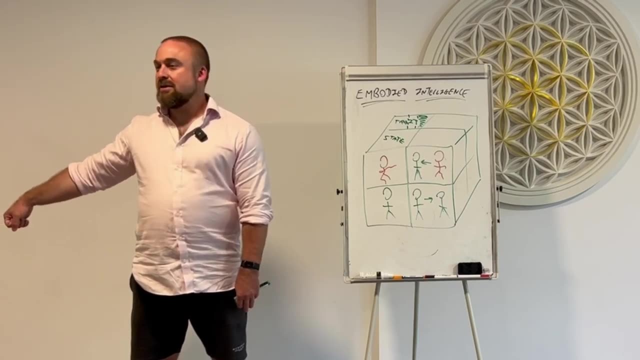 What will happen to me? Yeah, Who's? who's changed their embodiment through immersion? Has anyone like worked in a company where everyone was depressed, or worked in a, but moved to a town where everyone was funny? How did you change? I lived three years in Poland. 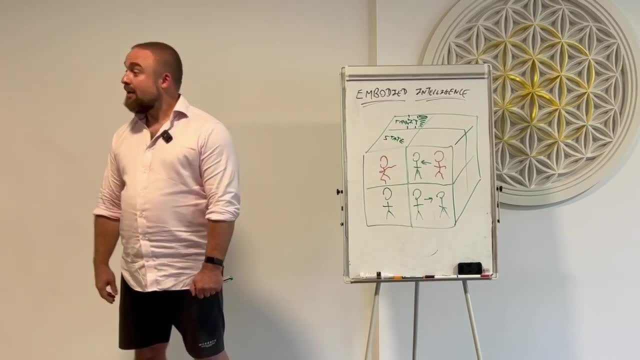 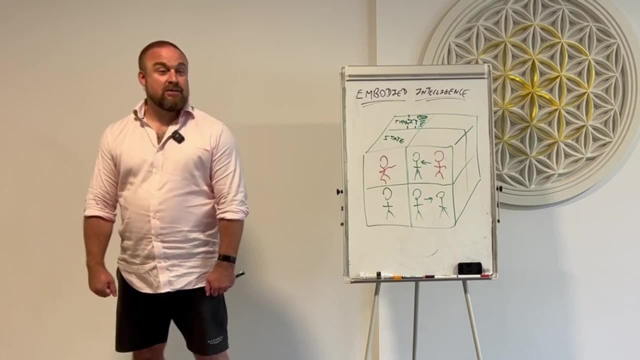 Oh, okay, What happened? My side of the language And I picked up the things that I like from them and incorporated it in my life. Great, And it can be more or less conscious. right, So you can live in Poland, living somewhere. 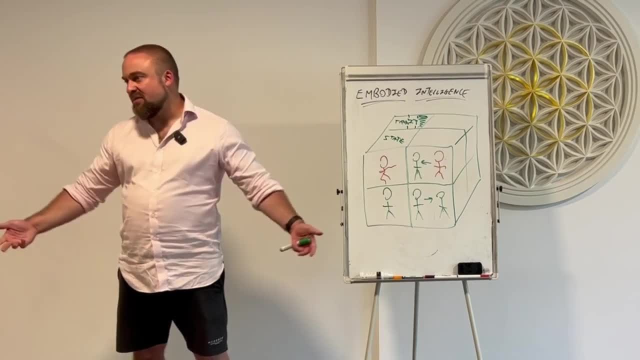 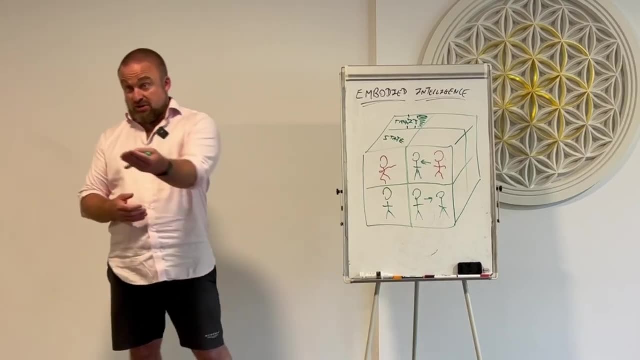 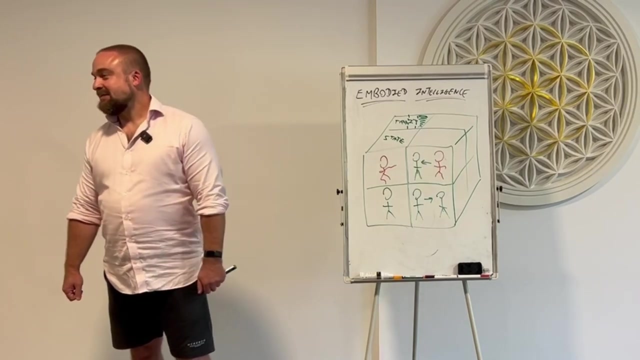 for three years is enough time. Living, going on holiday for a week, not so much. Language is like this as well. right, Like we have a look at the French speaking a Swiss. it has a feel to it. The way I spoke, English changed, Yes, Because they had an accent. Okay, And before I came, 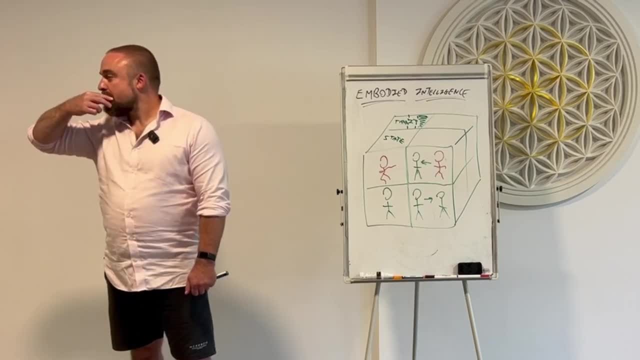 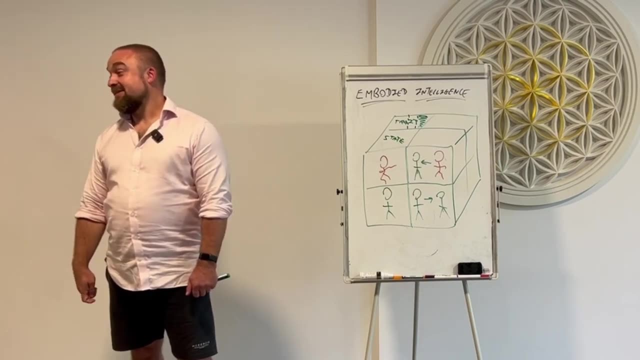 there my accent was different, So when I was speaking with them, I picked up more of their Polish English speaking accent so that I would be more understandable to them. Great, I don't know how you can speak great English like without the, like, the, the, the, the. 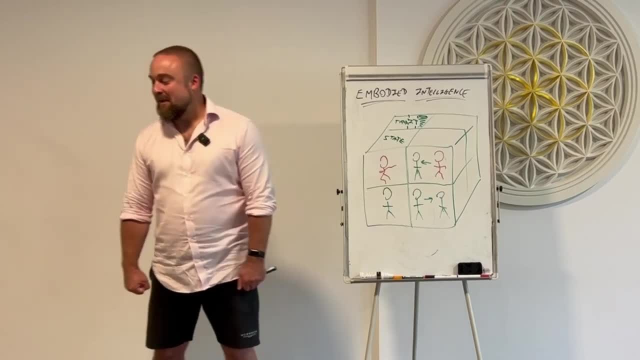 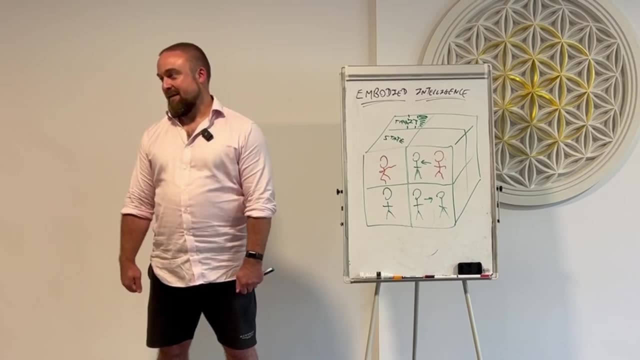 the accent. Yes. Then I started and I was cutting out some words, like they did, because then I would be on the same level. Great, We're adapting. And one day I was like: what are you speaking? Let's move on. 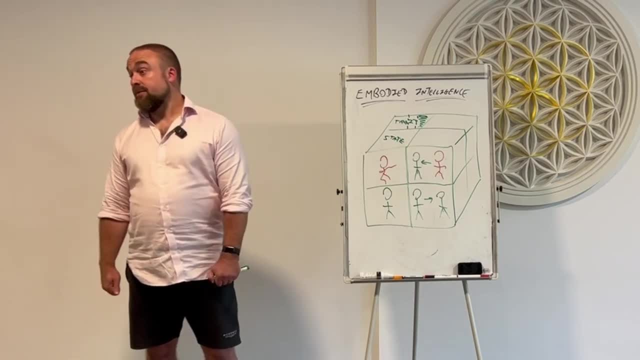 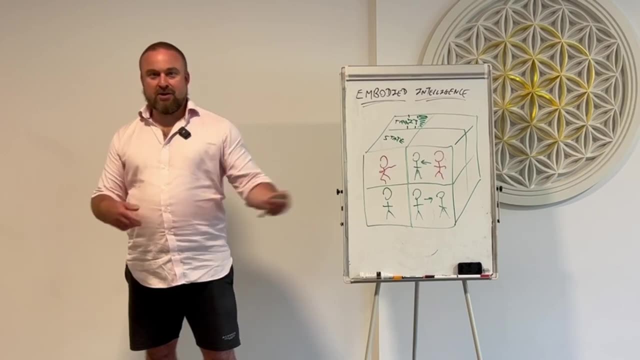 We're including a load of words. We adapt. My accent became more American because I'm speaking to people who learn English with Americans. My mom says I sound weird now You listen to old YouTube videos of me from like 13 years ago. I'm like: hello, my name is Mark, I'm English. Now I'm like: hey, buddy. 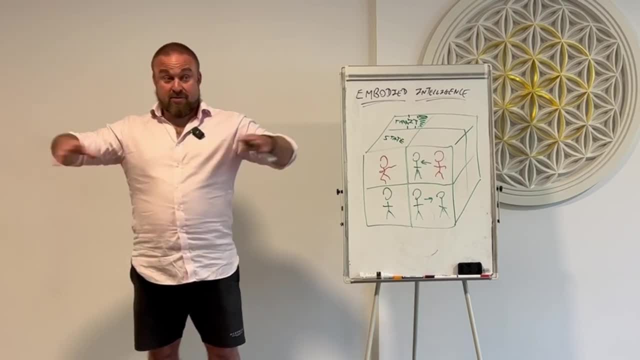 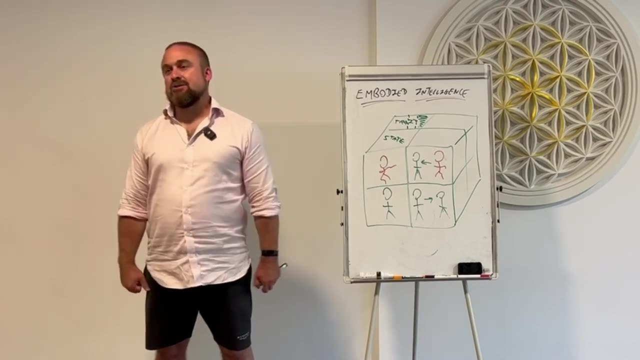 Shifts right, Like I'm spending 50% of my time around people who don't speak English as their first language. It shifts. So accent's an example, but your body has an accent. That's your embodiment. It's a nice metaphor, actually. 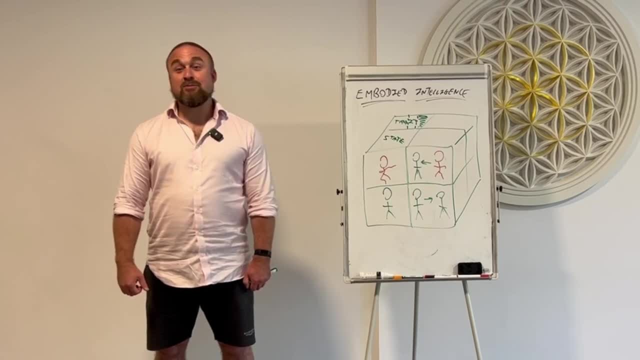 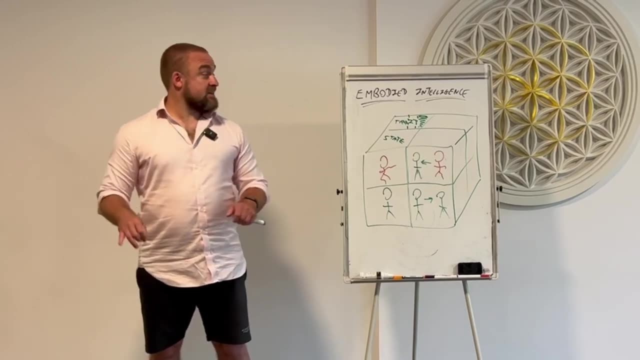 What's the accent of your body? Your accent of your body could be: I am sweet, I am nice. It could be I am tough, I am clever, And when it becomes a have-to, we're limited. If it's, I can be sweet, fine. 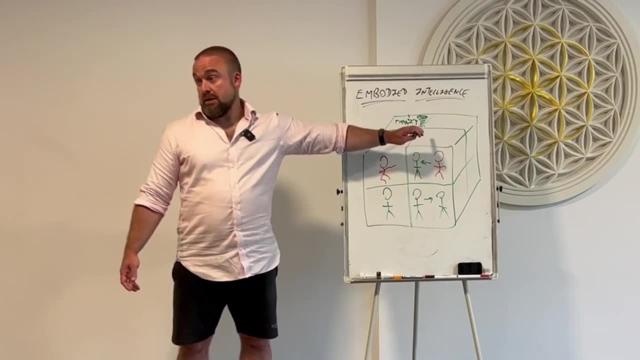 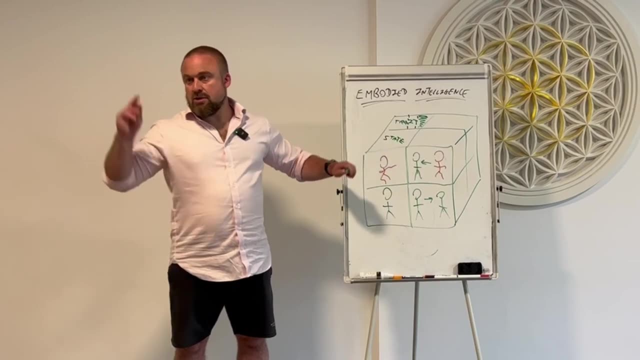 But if it's, I have to and I can't be tough, then we have a problem. So the basic journey of embodiment is becoming aware of states and getting better at shifting them. You don't have to, you can't, just change. 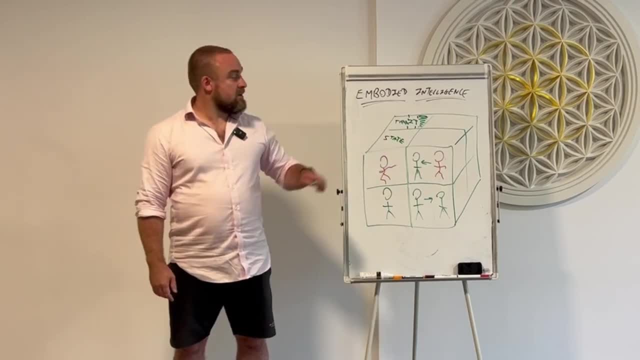 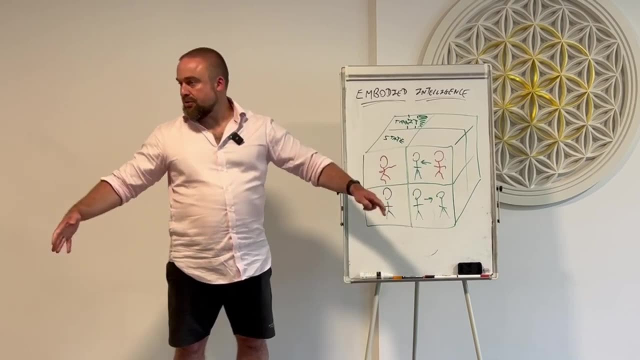 but you can get more influence, more leadership, self-leadership, Becoming aware of traits and developing more range. So people who study with me for a while, they develop practices, they build their range. Great, so we have self-awareness. 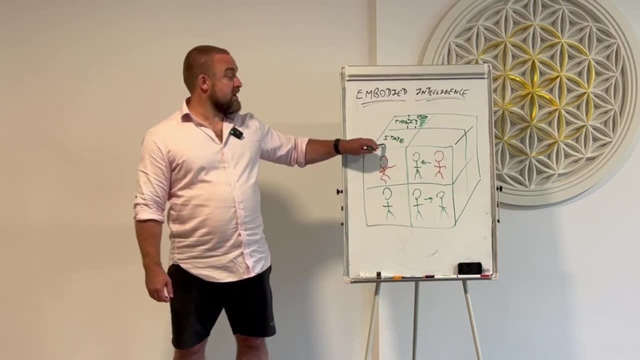 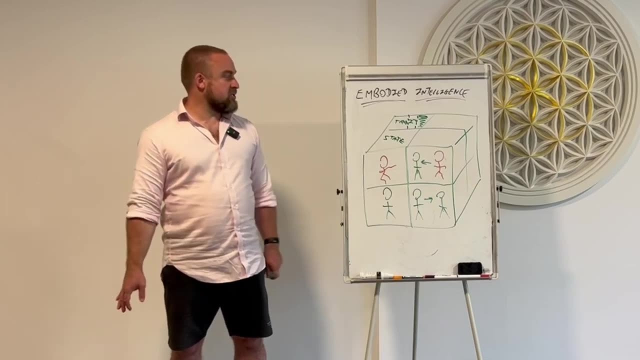 and then we have this we could say self-regulation, So it's regulating states and changing traits. So I just described this half of the cube- You with me- As facilitators- super important. What state am I in Self-regulation? 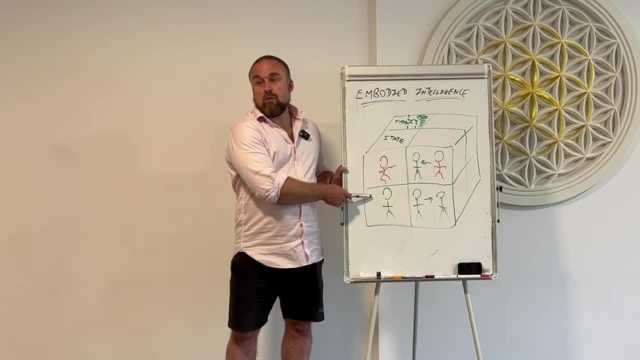 So awareness and choice, Or we could say: what is and how you want to be. Okay, this is you shifting, making a choice. self-leadership, self-management- there's different words for it. If I'm in business or something. 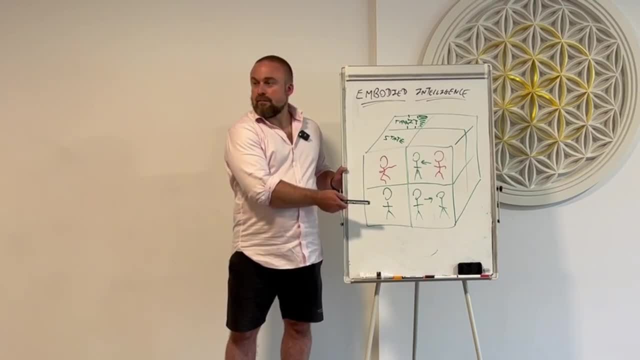 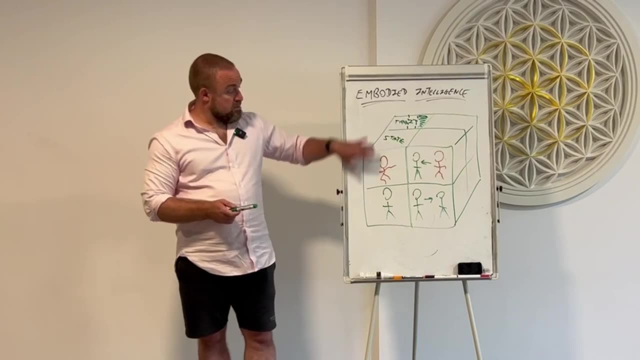 I say self-management, Yeah, Okay. so we've got awareness and choice, Very simple, Short-term and long-term. So that's what we've been playing with for the last half day As a facilitator- super important. What state are you in? 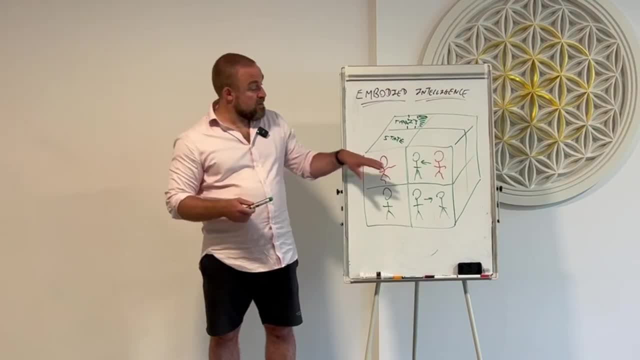 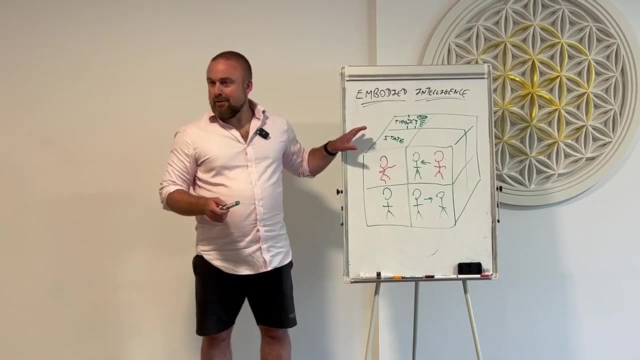 when you're facilitating, Because you will be influencing other people. I'm going to come to that in a minute. Yeah, Can you manage your state? Sometimes I turn up for training and I'm in a real bad mood. I read something on Facebook: 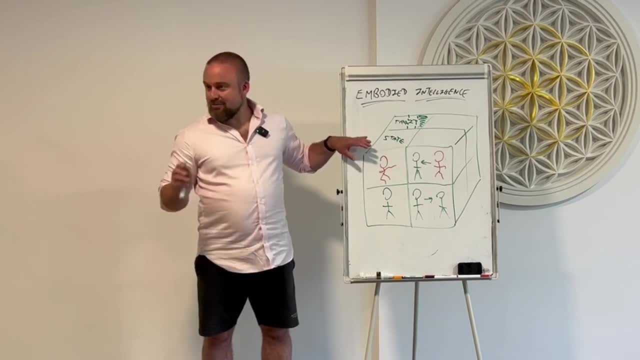 two minutes before I went, you know It's like: okay, I need to regulate my state. Also, knowing, even just knowing, your traits. I know I'm a certain type of trainer. I talk to a corporate client. They're like: 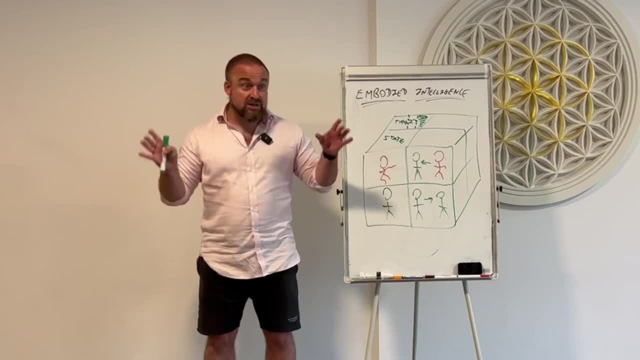 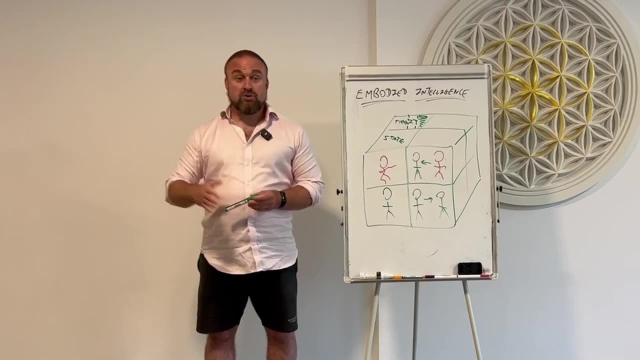 hey, can you come to a HR convention And I'm like I am going to make dick jokes, Is that okay? Yeah, I know my style is, humor, is, provocation, is direct. Sometimes that's good, Like you saw me coaching a guy earlier. 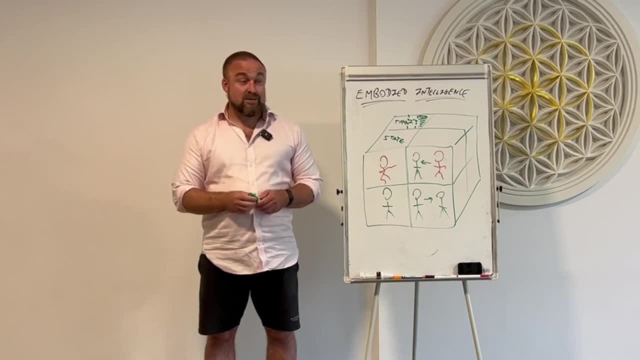 I think he liked the fact that I was quite direct. Other coaching clients. I'm like: yeah, maybe we're not a good fit. You're someone very delicate, very vulnerable, You don't like humor, You take life seriously, You don't want to be challenged. 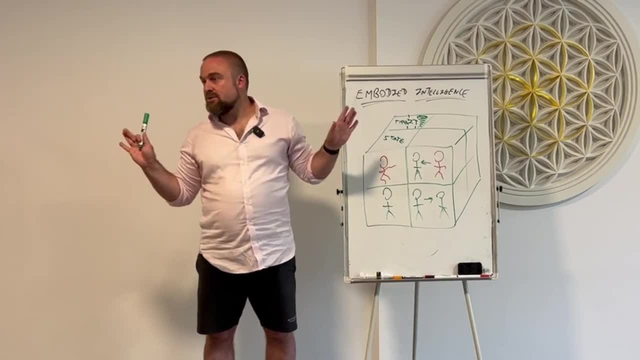 Yeah, I know this is my trait, So maybe I don't want. maybe it's not a good fit as a coach. I know someone: why don't you work with Ava? She's much nicer than I am. Yeah, So just the awareness. 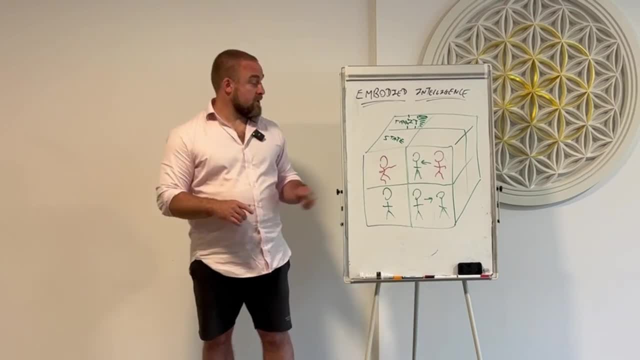 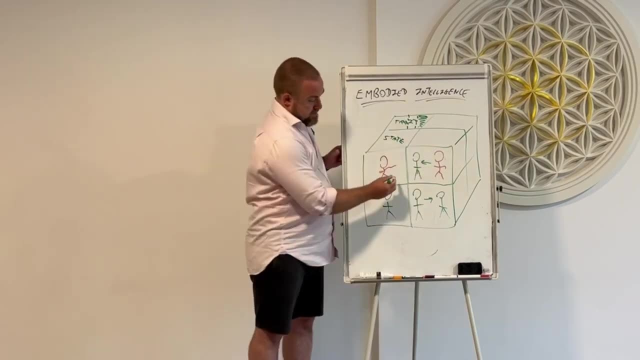 is already useful. Okay, All right, Let's go to the other side. So this is a facilitator. This is super important. In a way, this is the direction, So we can't regulate ourselves until we know about ourselves, If we're relatively regulated. 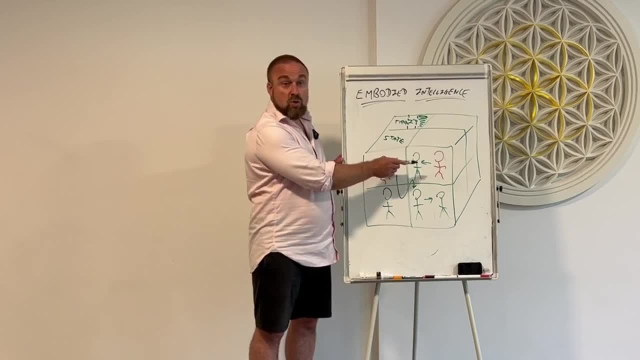 we can listen to other people. So this is social awareness. Self-awareness is social awareness. Yeah, So we're aware of ourself. If we're aware of ourself, we can get our shit together- Technical term: If our shit is reasonably together. 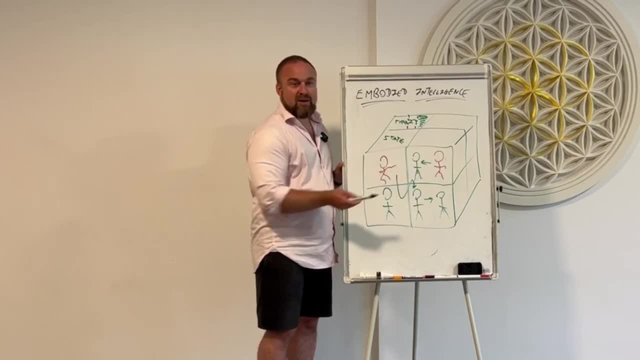 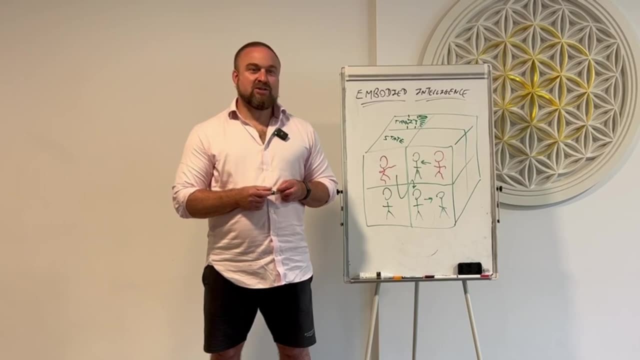 we can be aware of other people. Yeah, Notice, when you're like having a panic attack or you're really angry, you're not very aware of anyone else, are you? You with me? Think of the last time you were really stressed and pissed off. 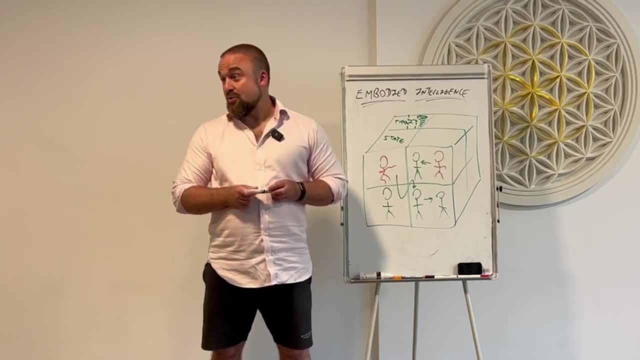 Were you like super sensitive to your husband's needs? Yeah. Were you like super aware of your children? Probably not. You were like too much dysregulation, Yeah. So if we're regulated enough, we can be aware of other people. 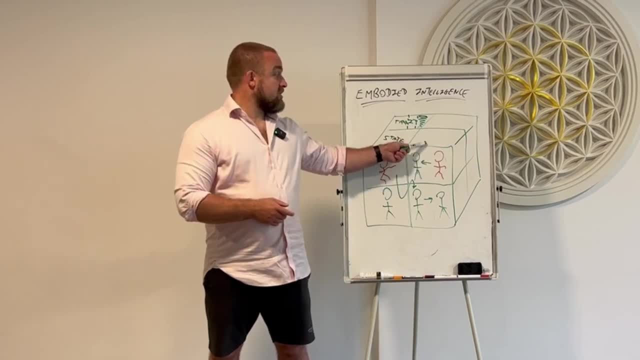 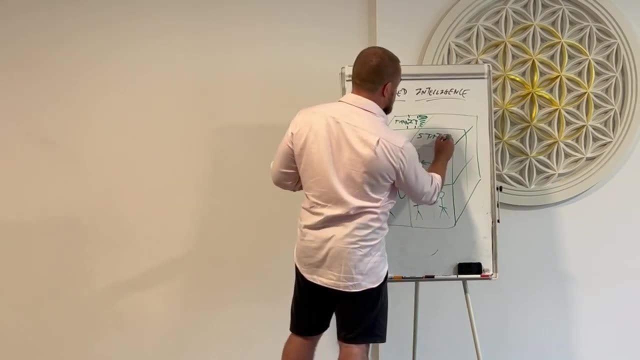 Hey, are you okay? What's going on? What are we aware of? State and trait? Same thing again. Yeah, So I can be aware of someone's state. How do I do that? How do I become aware of someone's state? 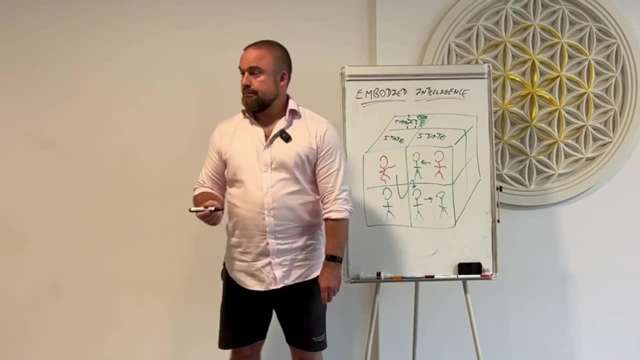 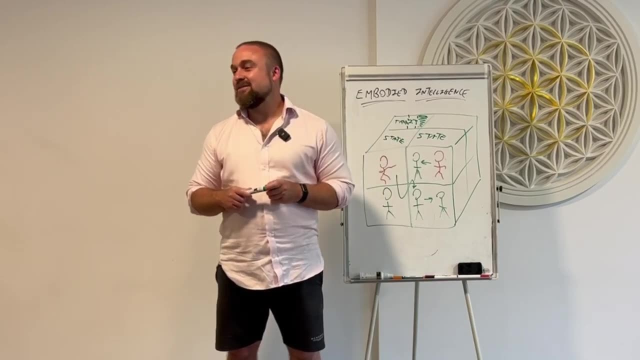 If I want to know how Ava is right now, what can I do? Okay, Magic, we could ask. That's how we get inside the subjective box. What else can I do? What? Yeah, I can look at her body language. 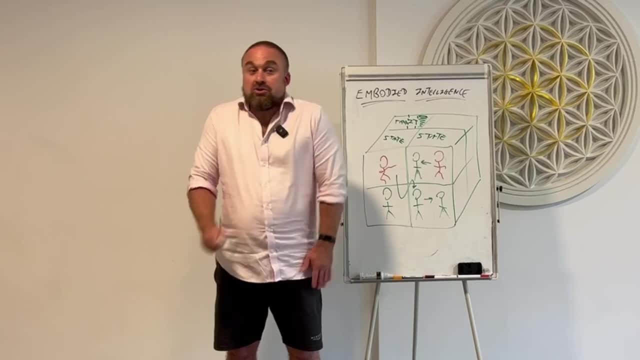 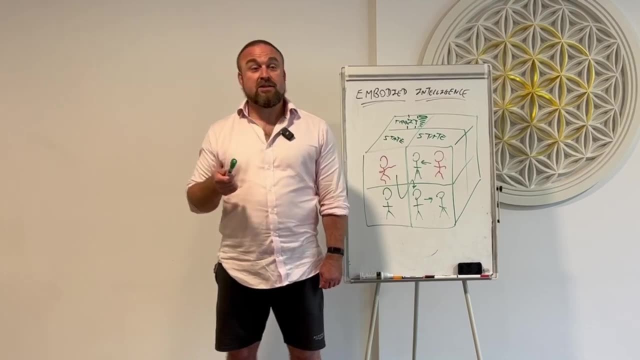 How's she sitting? What's her blink rate? How's her heart rate? Are her shoulders up here? It's common sense, right? So I can do that actually two ways. One is I can observe, The second is I can empathize. 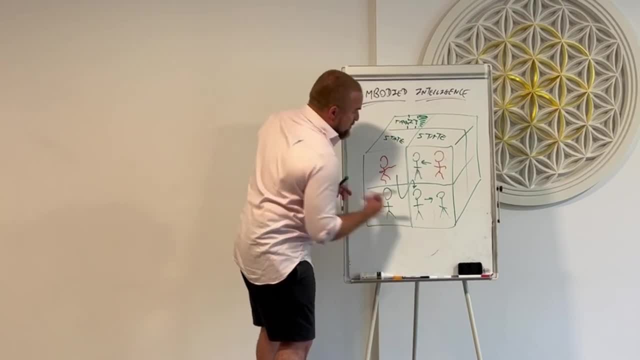 So in a way, we've got this sort of little arrow back here, Right. So observation is just cognitive. I can go. okay, she's blinking this much, She's breathing this much, She's got her legs crossed, She's got her shoulders. 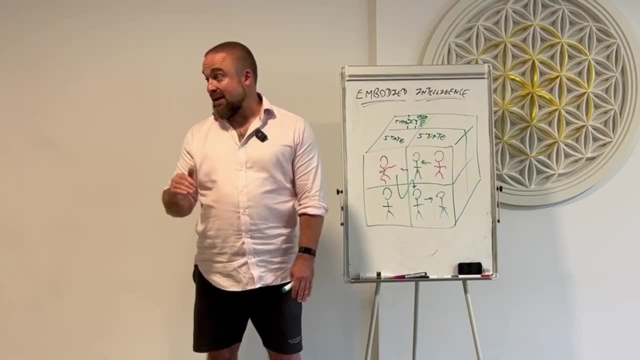 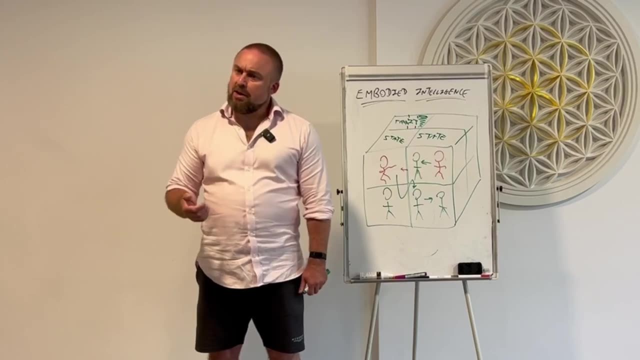 tight or not tight. That's just observation. It's cognitive And I have to be relaxed to do that. The other way is empathy. I can look at her and go: okay, oh, I feel really sad when I look at her. 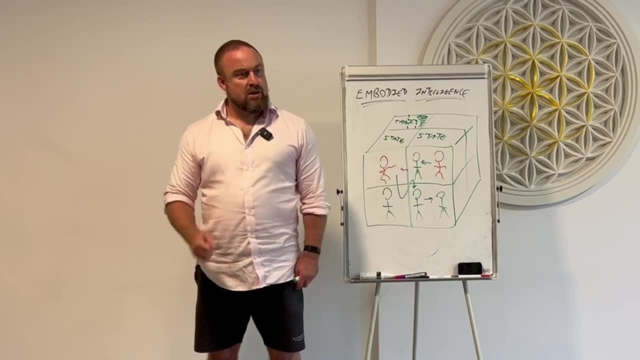 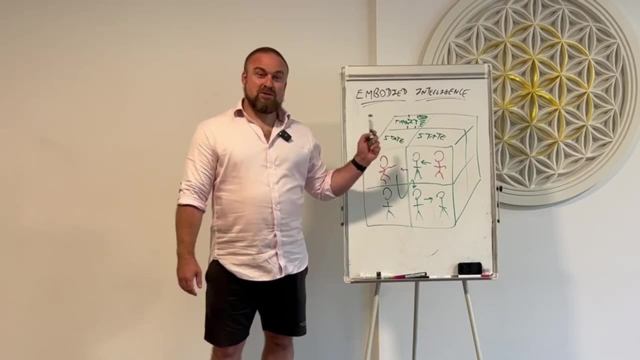 Or, oh shit, I'm getting angry. She seems upset. Look, I'm noticing I'm dysregulated when I look at her. Yeah, So of course, if you're not a psychopath, you will do this naturally. What's the danger? 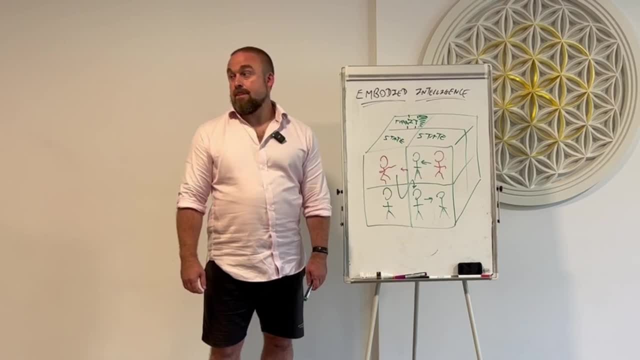 for us as facilitators in this Right. So if she's dysregulated I can get dysregulated, Like I gave the example of the mom in the supermarket yesterday The kid's having a tantrum because they can't get the candy. 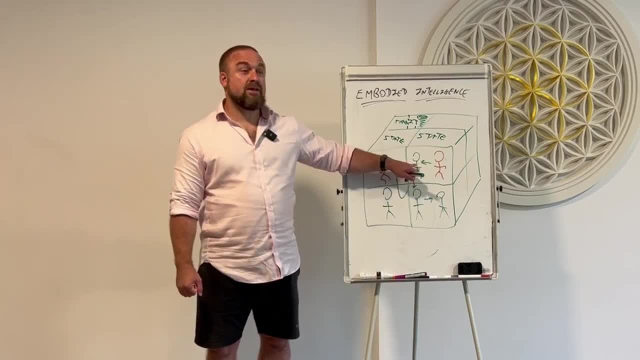 Right, The mom is regulated enough that she looks at the kid and goes: okay, the kid's upset Pretty fucking obvious actually with the kid. She can then regulate the kid. So the last one here is social leadership. Yeah, 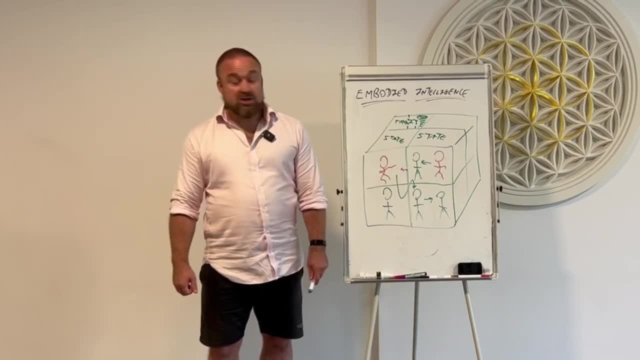 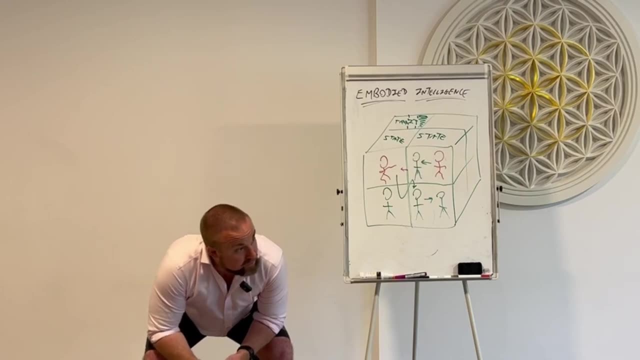 It's regulating others, helping others, supporting others. She had her shit together enough, this mother, that she could say: hey, I know you want the candy. It's okay You're not going to get it, but I still love you. 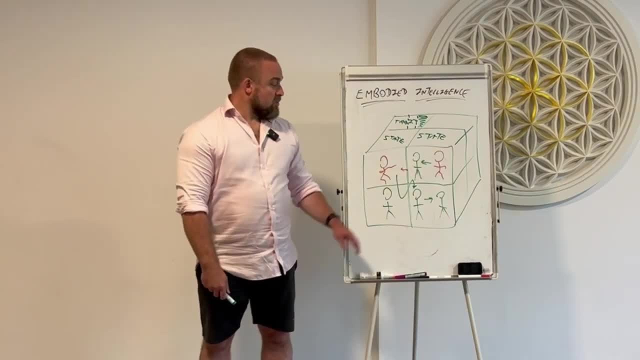 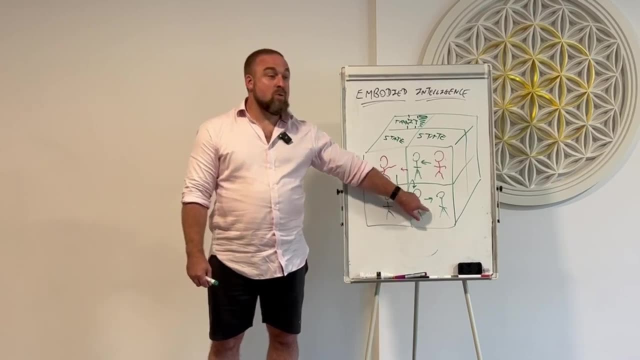 You were doing this with your, your child yesterday as well, right, So we naturally do this. We do this with our friends. Hey, there, there, It's going to be okay. Yeah, As facilitators, this isn't always down-regulation. 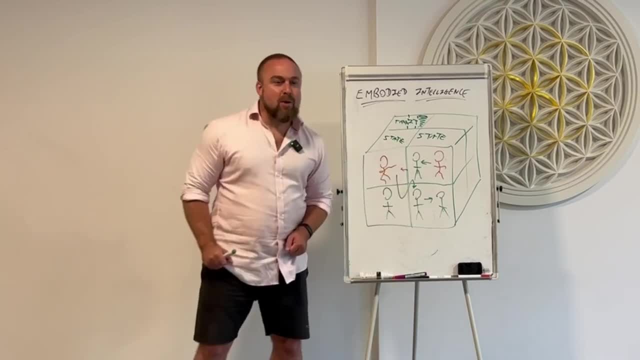 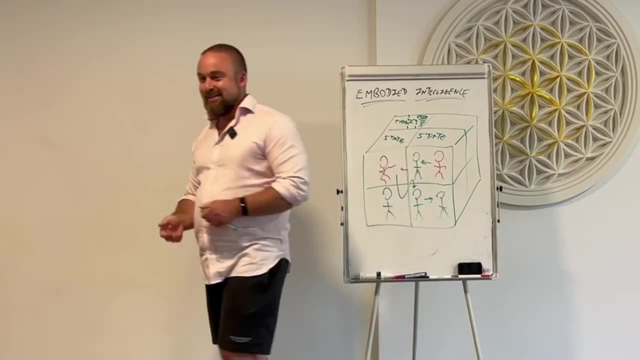 Sometimes it's up-regulation, Okay, Hey, okay, Welcome to the training. My name's Mark. How you doing? Everybody okay, High five, It's American style. Yeah, It's up-regulation, Or I make a joke. 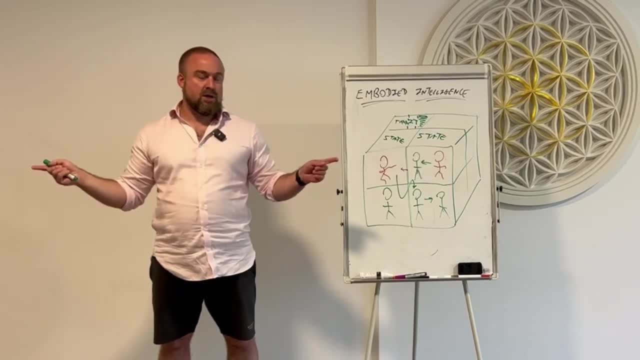 You've seen me make different jokes, right. When I was doing like the dick-sized joke yesterday- Don't ask YouTube, Okay, When I was doing that joke, everybody woke up. You were like: ah, this guy's funny. 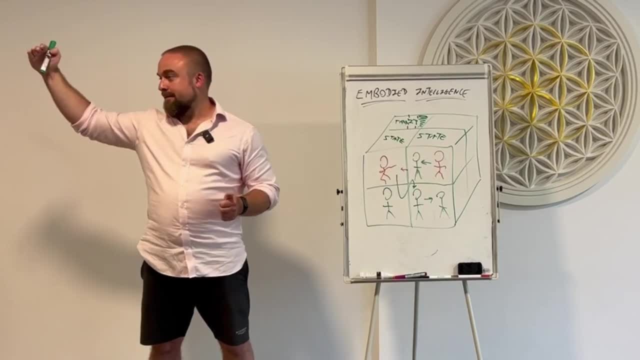 What the fuck? I can't believe he's saying this. Right, I was up-regulating you, Yeah. The main way we have to work with, though, is what? Not just jokes? What's the main thing we have to work with? 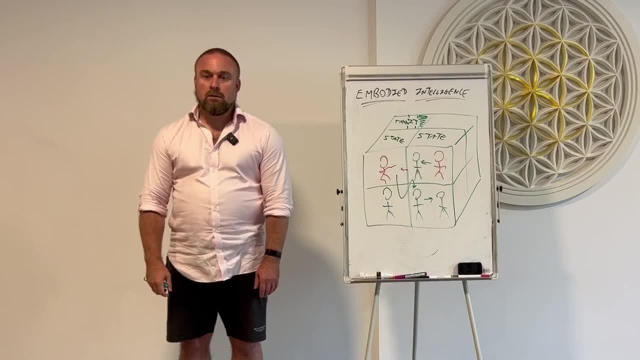 My own body right? Hello, I am going to motivate and energize everyone. I am the inspirational speaker in the company. You're laughing, right? This is ridiculous. Like I have to be energized, right. Like I have to come in. 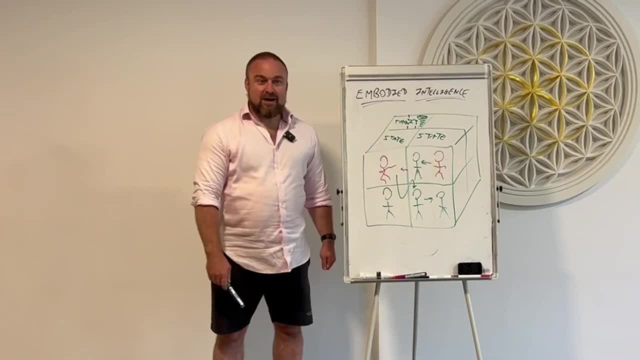 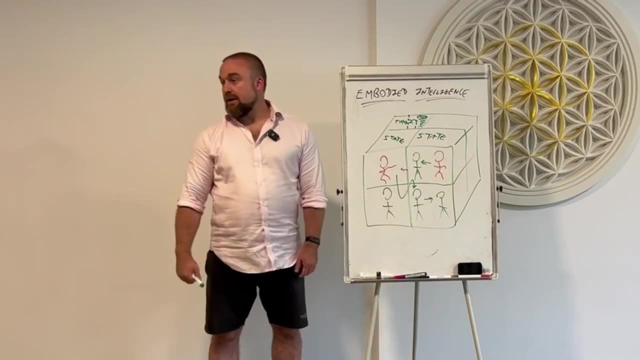 I might need to self-regulate myself. I might have to go outside, take some fresh air, walk around, drink a coffee. I can wake myself up, Yeah, So then I can do you. I can lead the group, Okay. 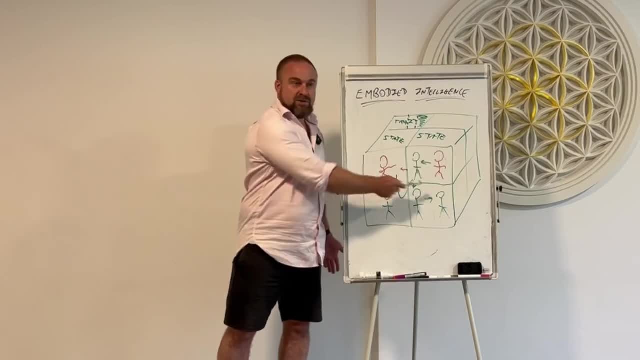 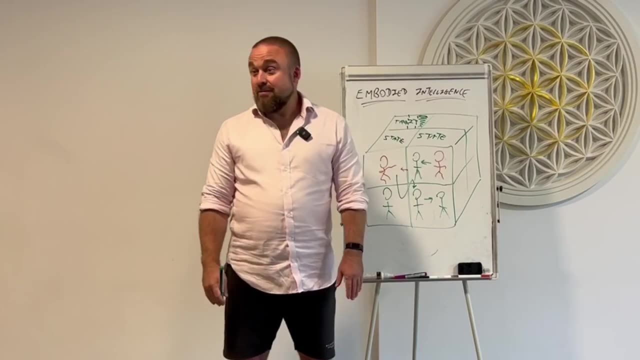 So if I'm not aware of my state, what the hell am I influencing? Earlier I gave that example of saying I'm marking you. You know, Like we're rubbing off, We're contagious. So first of all is awareness. 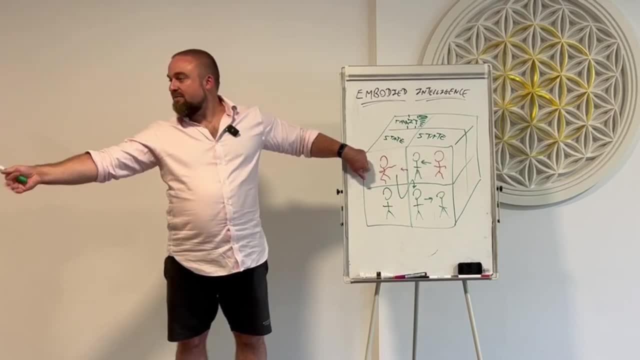 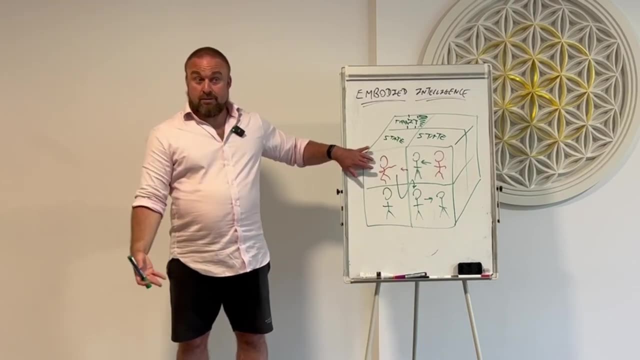 What am I spreading to you right now? Yeah, I'm infecting you, I hope with enthusiasm and focus and inspiration. I hope I'm doing that right now, But if, if I'm giving you something, okay Now, it's not as simple as that. 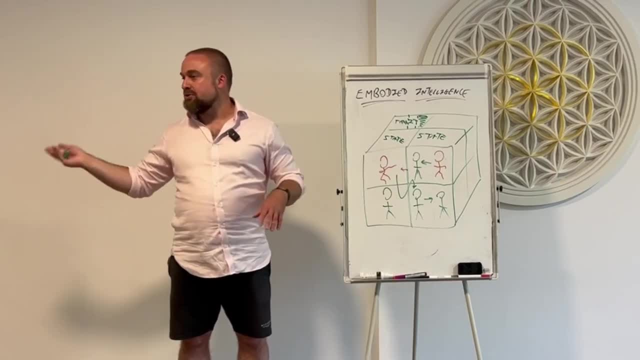 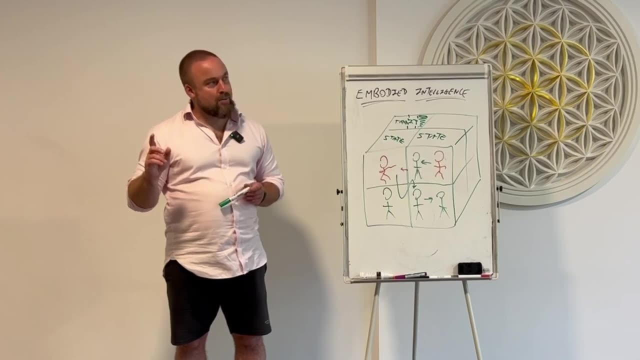 because you could be having a reaction. I could, you know, have a trauma pattern that reminds you of your school teacher: Blah, blah, blah, blah, blah. It's not quite as simple as There's. How much do I want to go into this? 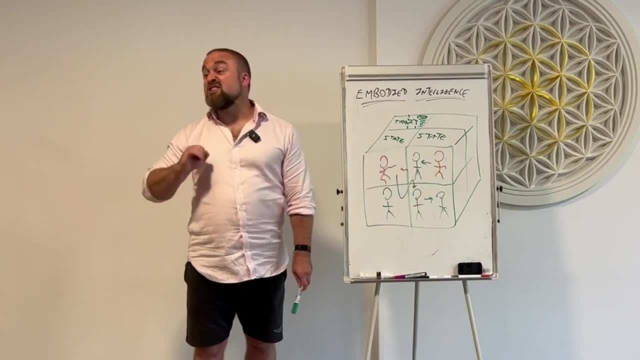 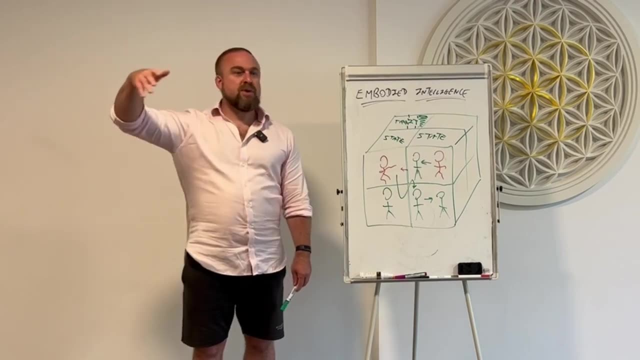 There's a few principles here. The most simple one is: just contagion. Your students become what you are. That's the simplest principle. So if I'm energized, you'll be energized. It doesn't always work that way because you have other factors. 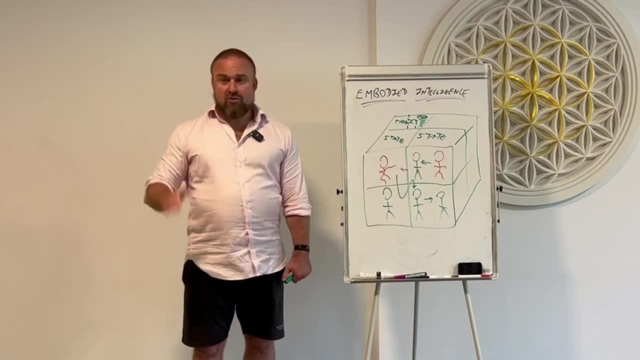 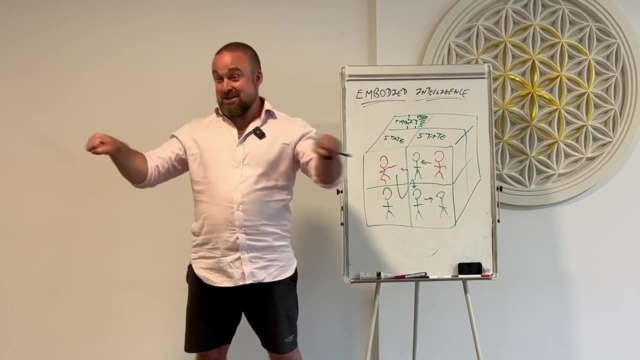 Things like polarity. Yeah, I could really dominate you and make you submissive. Some of you are like: not me bitch. Yeah, So you're actually going to. that's actually going to make you less submissive. Some of you actually will go. 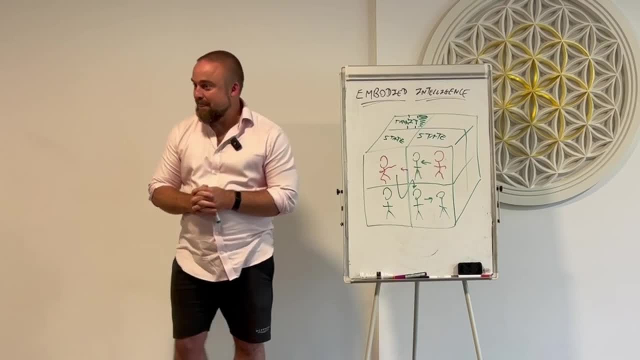 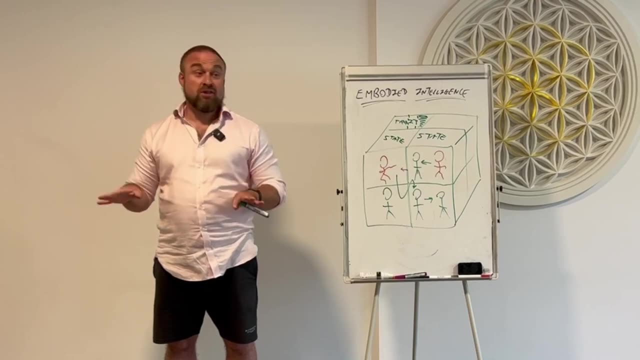 okay, Okay, daddy, Yeah, Does it make sense? That's polarization. That's what happens sexually. by the way, polarization, Yeah, It's not always in sexual context. that's a good thing In a training context. 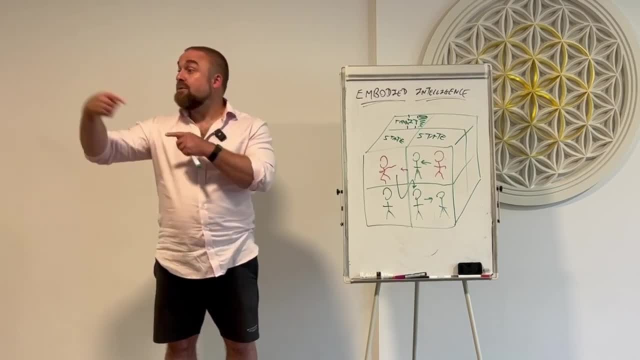 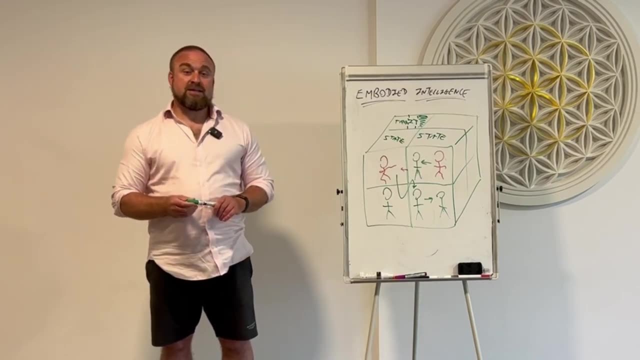 maybe. Yeah, Do you understand polarization? So you become the opposite of what I do. There's another piece here which is role-taking. This is systemic, So it's like, okay, let's say everyone's trying to be the funny one. 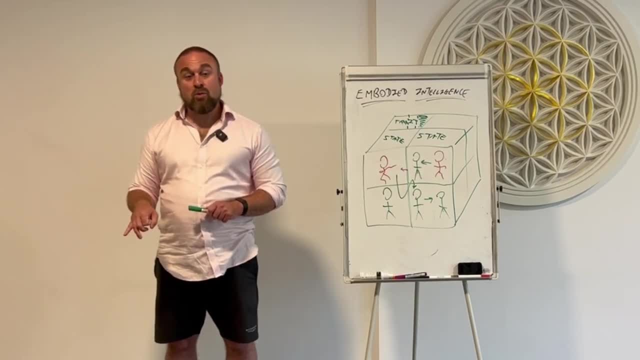 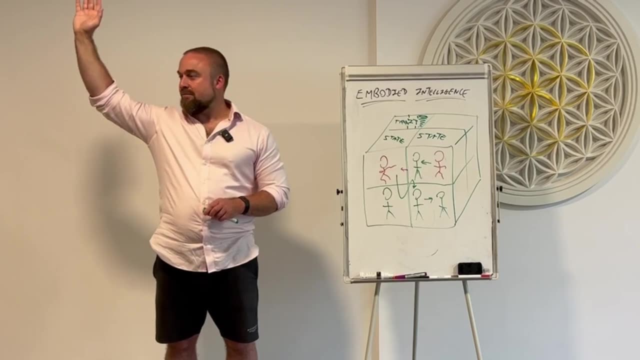 That doesn't work. So what will happen is, systemically, we'll decide who's the funny one, Yeah, Or let's say, everyone who's like caring looks after people, kind of a caregiver. Ava's definitely got that right. 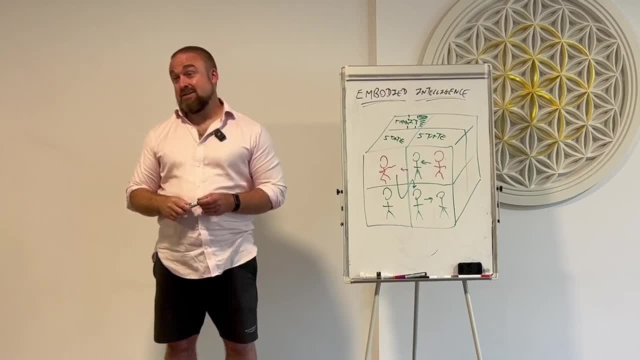 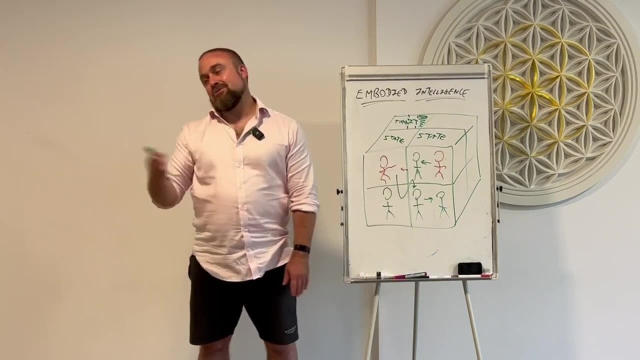 If you all try and do that, it sort of doesn't work. So this is systemically. we're going to like unconsciously decide: okay, you're the mums, Yeah, You're the caregivers, They're not. literally. 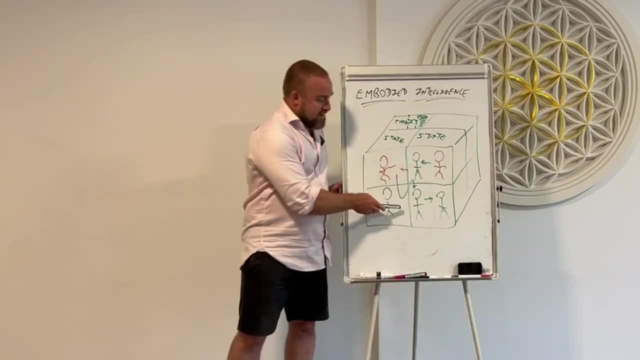 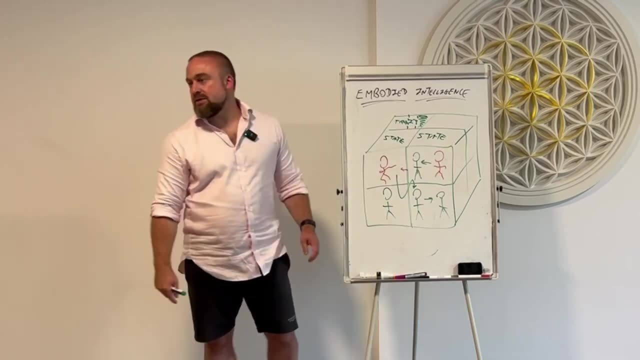 Does it make sense? So it's not. this isn't quite as simple as just infection of just contagion, But contagion is the general rule. There's a few more possibilities, Yeah, So that's it As a facilitator. 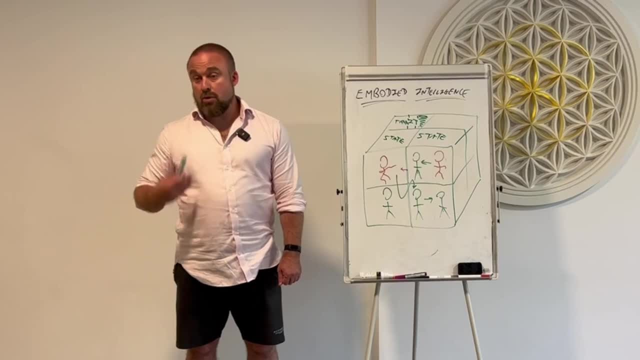 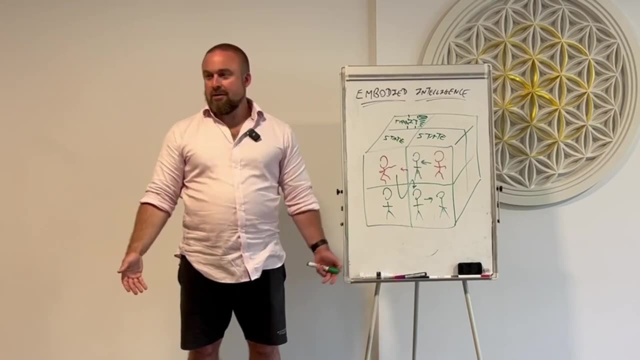 Yeah, Yeah, yeah, yeah. So voice, we have our body, we have our voice, we have direct methods. So I could say: okay, everybody, everybody, high-five each other. That will up-regulate you Like. here's one I use. 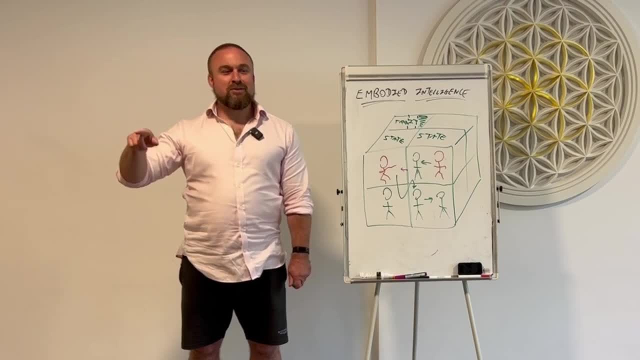 Okay, turn to the. you look a bit sleepy actually. So everyone, turn to the. look a bit sleepy. I'm observing you, right, I'm seeing a bit of this. I'm also feeling that in my own body, Like it's becoming hard work for me to teach. 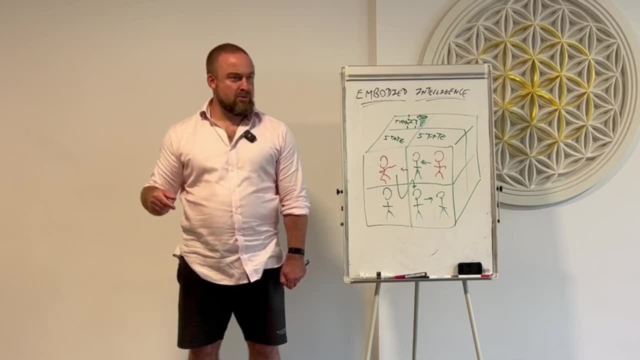 Why is it hard work for me to teach? Because you guys are down-regulating me a little bit, Not too much, but a little bit. That's fine, That's my job. So I want to up-regulate you now. I could do that with my tonality, right. 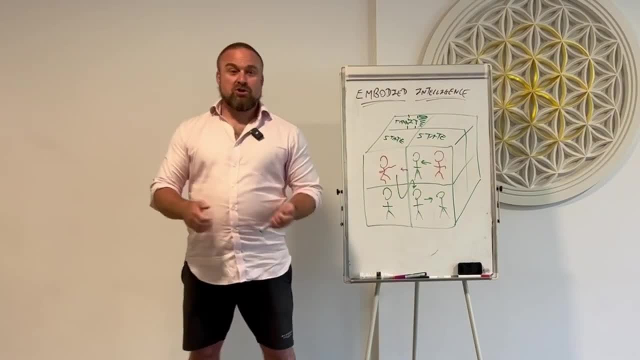 I could be like hey, up and down, woo. and yeah, yeah, Yeah, I could do it with a joke, Yeah, I could do it directly. So everyone turn to the person next to you. The smaller person hits the bigger person on the hand. 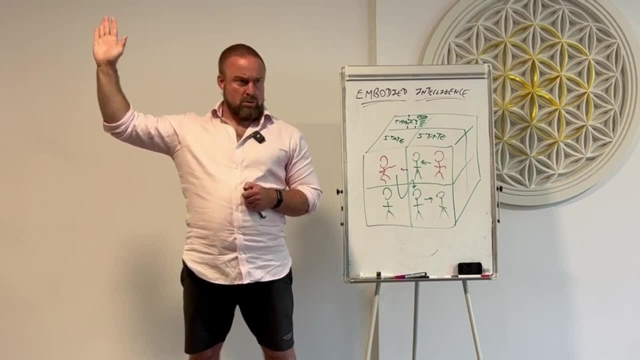 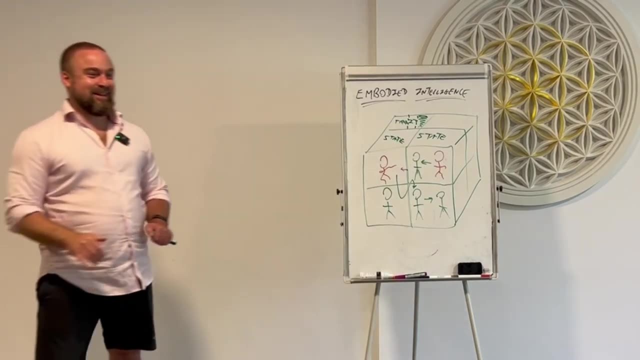 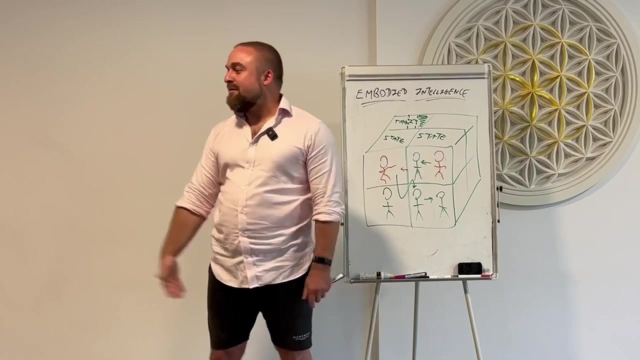 hard enough, so you make this noise. Ow, Does that make sense? Turn to the person next to you. Smaller one high-fives the bigger one. Smaller one hits the bigger one. Yeah, Not with a fist, Fucking with a fist. 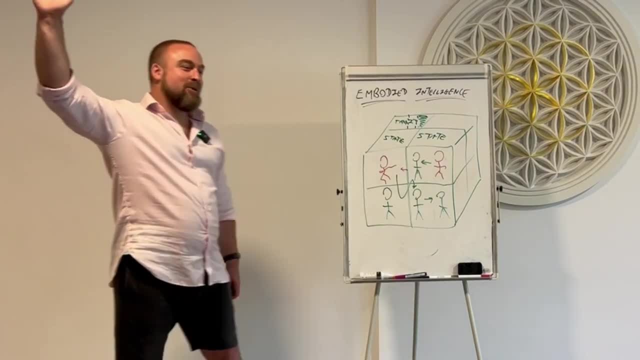 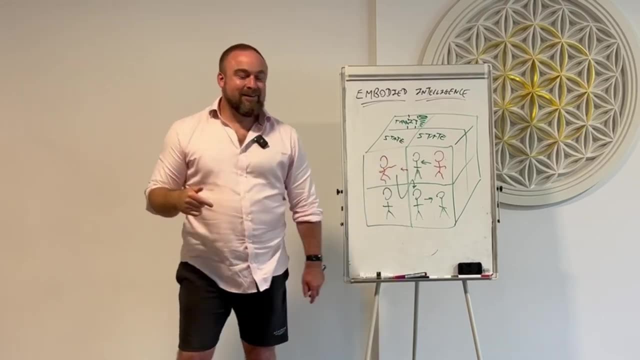 What is this Croatian bullshit you're doing? Okay, pause, pause, pause. That's good. I can't shut you up. That means you're up-regulated, That's good. Yeah, Do you feel the difference now in the group? 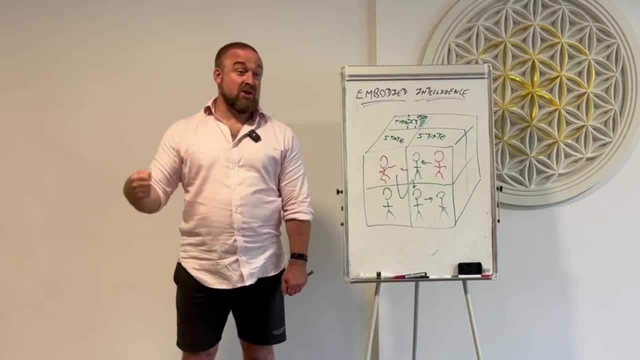 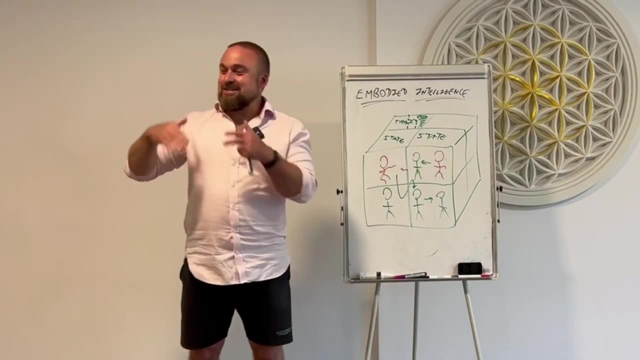 So that was very direct. By the way, the Croatians started punching each other. That was a joke. I just up-regulated you with a little bit of Croatian racism. There we go, So do you see how it works Right? 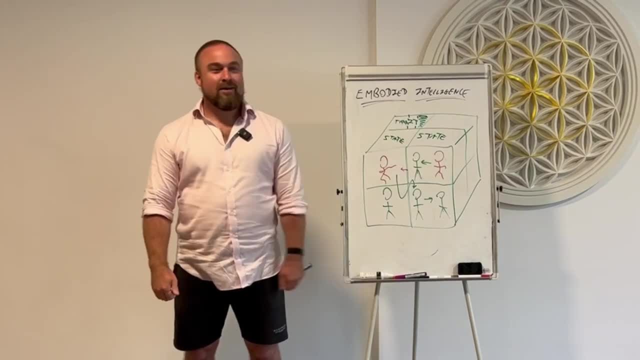 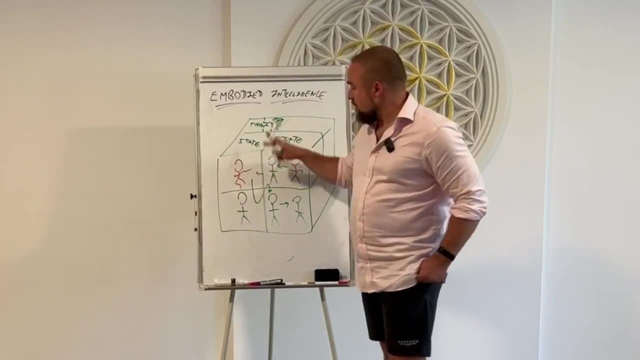 So we're doing it directly, We're doing it through voice, We're doing it through humor. Okay, Different methods, Okay. So this is it. It's very simple. As a facilitator, you're becoming aware of yourself, your traits and your state. 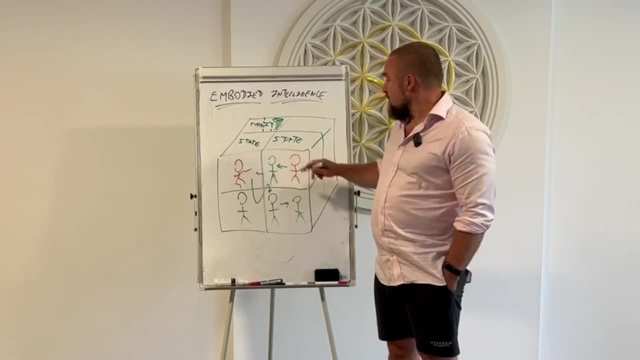 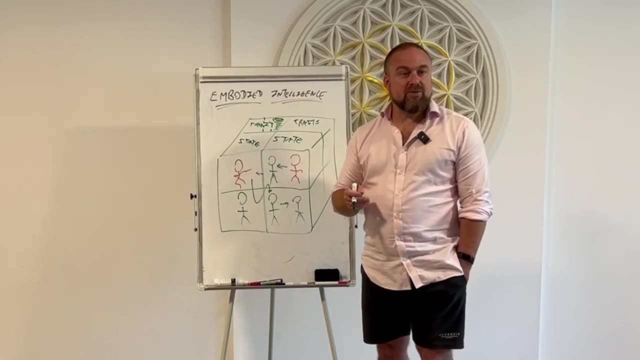 You're regulating them. You're building range. Yeah, You're becoming aware of traits and states. So traits you're probably observing. You know you're learning some models, Like I'm teaching you some things. right, These models can be silly. 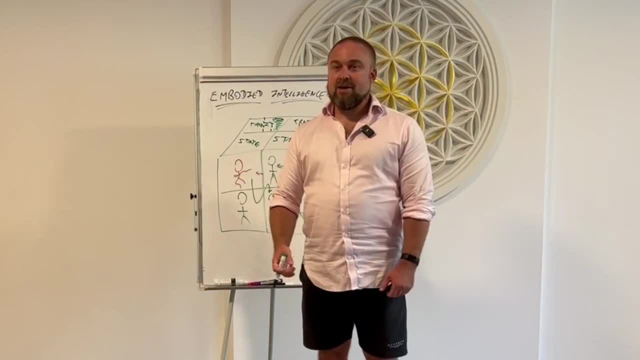 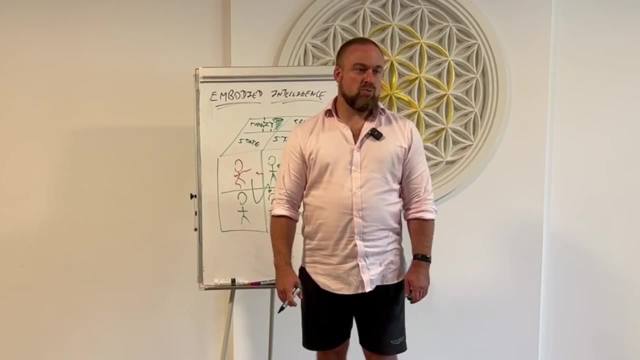 Like: are you Gary or are you Shanti? They can be. you know, you're a shark or you're a sheep. They could be four elements model. They could be Myers-Briggs right. Extroverts, introverts walk differently. 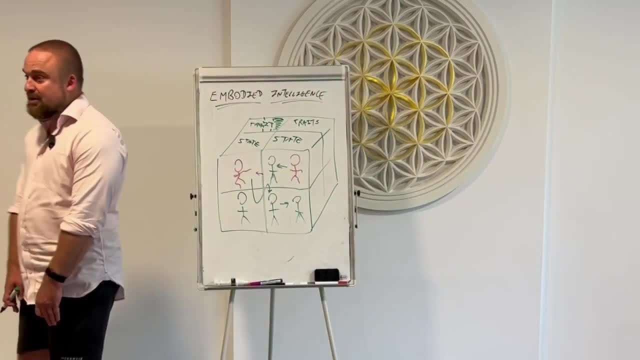 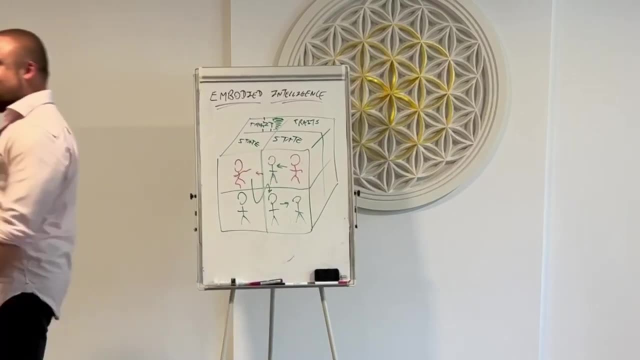 Introverts have smaller steps, Their arms move less. Yeah, Like, imagine, like a little Japanese geisha. Yeah, Extroverts, you know, their legs move, their arms move. It's a different energy, Yeah, Different monument. 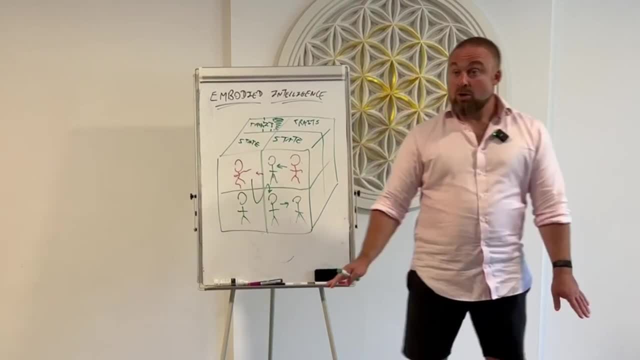 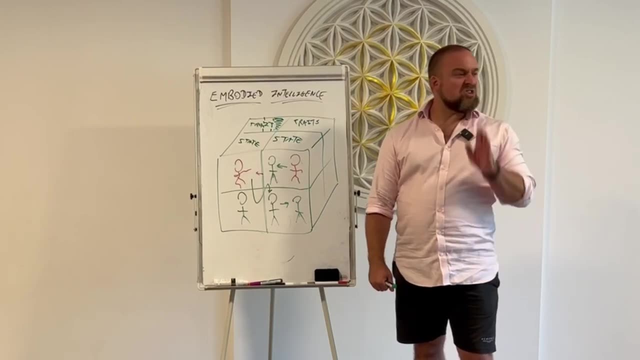 So you can learn to observe this and get better at this. I love people watching. You love people watching. There's a trainer Like: sit at the train station. Me and Miri do this. We make up stories about people. We judge the shit out of people. 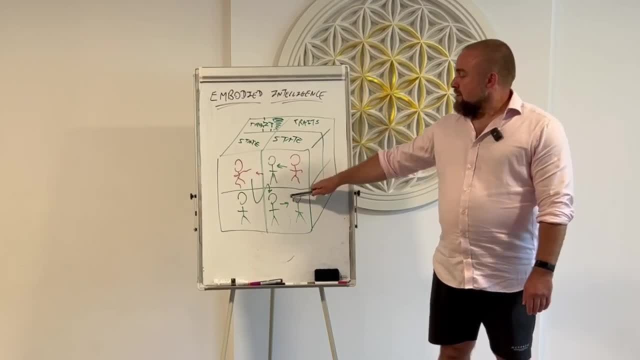 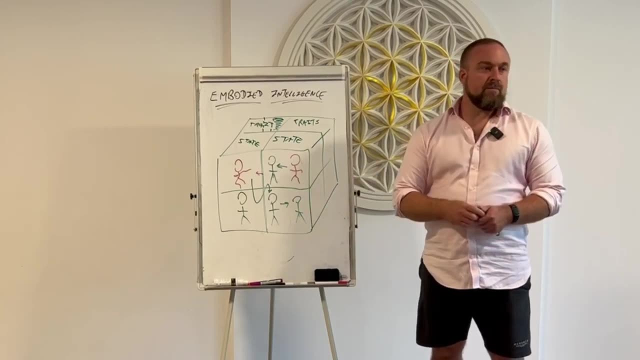 Yeah, Just making up stories. How do you influence people Using the rest? All right, You influence people by self-regulation and then direct methods as well. So this is body facilitation. This is what we're studying. Yeah, We'll end the video in a minute. 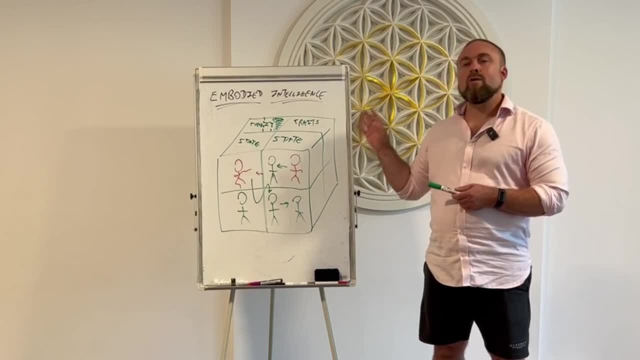 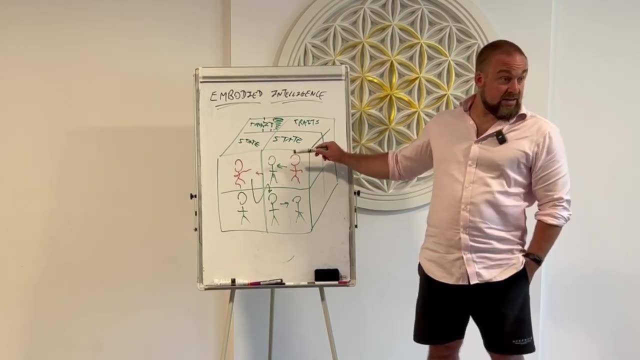 But the thing I want you to discuss in pairs is: like what are you already good at Make sense, Like some people are just talented. Some trainers are just really empathic, really sensitive. Yeah, Maybe personal cultural trauma. Some people are just really funny. 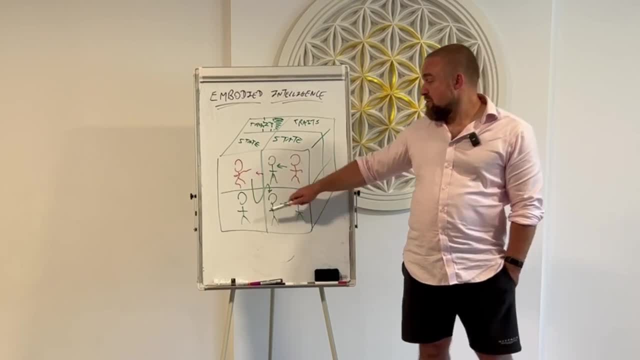 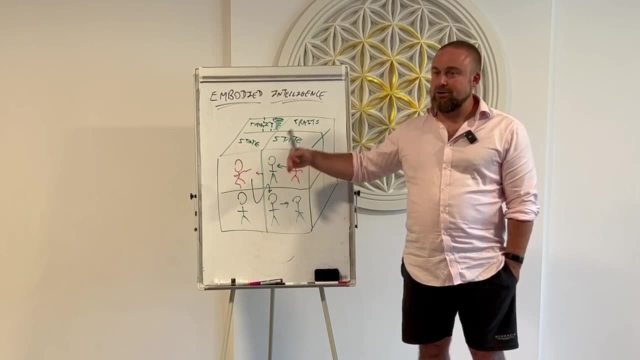 They've really got the humor piece down. Okay, Some people are really sensitive. I'm not very well self-regulated. Yeah, I'm like ADHD recovering alcoholic. I can like just about regulate myself, but I'm not like great at it. 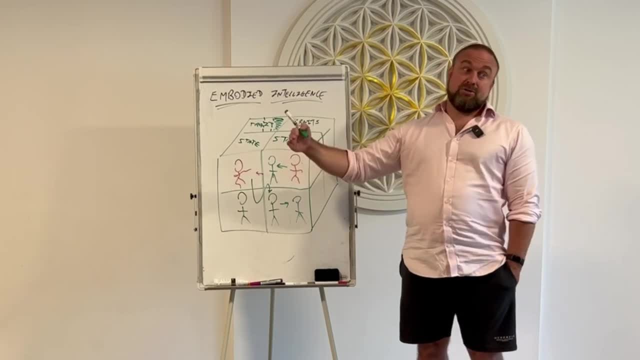 I'm like adult level now, but I'm not like a genius at this shit. Yeah, And it's probably way better than me at this. Make sense Emotional awareness. I used to be terrible at it, Eh. 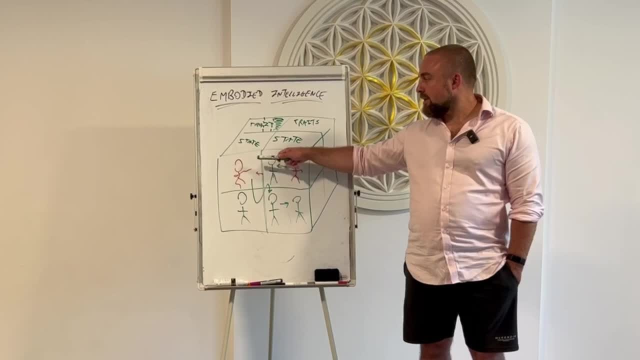 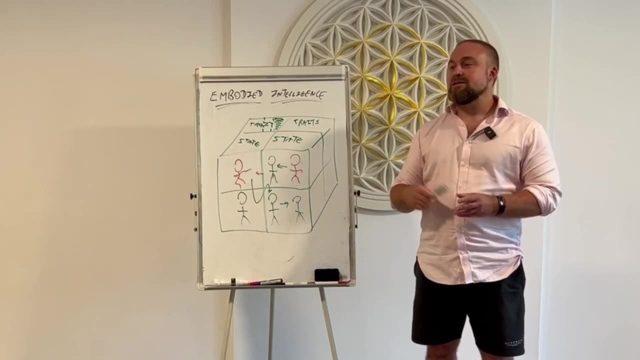 Lived in California for a bit. Now I'm like, yeah, I'll tell you about my feelings. Okay, All right, Cool, Cool. So just in pairs. where do you think you're kind of talented? Where have you learned something? 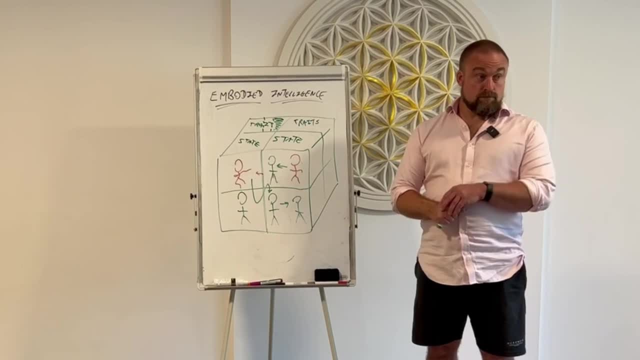 Where maybe is there some room to improve Cool. 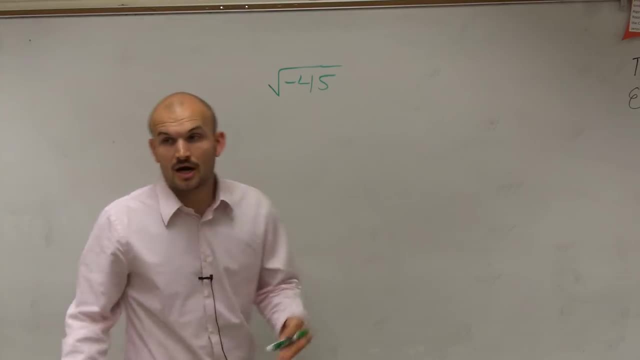 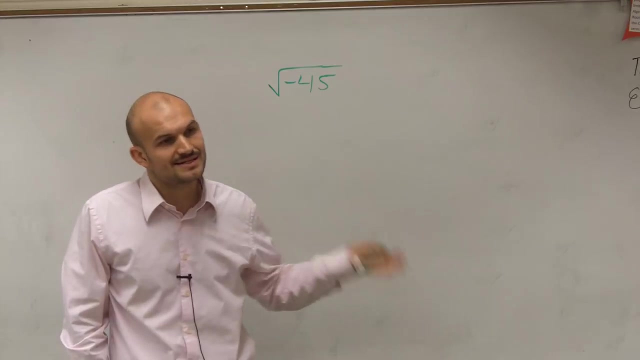 So we talked about how you can take the square root of a square number, but what do we do when we want to take the square root of a number that's not a square number? Well, remember, we need to simplify the radicals, So hopefully you guys remember what square numbers look like. 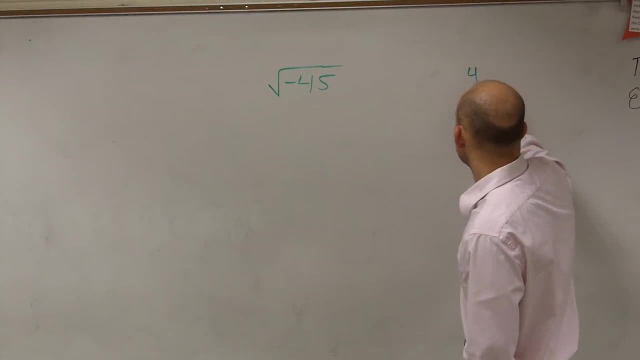 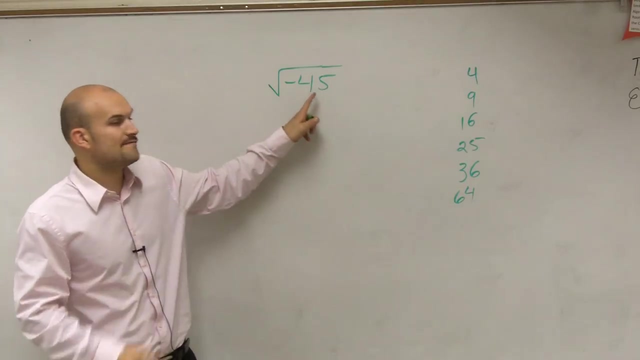 And this is the easiest way I like to write. I like to simplify radicals. I write down the square numbers all the way up to what's in my radicand. So, to simplify radicals, what you want to do is you want to factor your radicand by one of these square numbers. 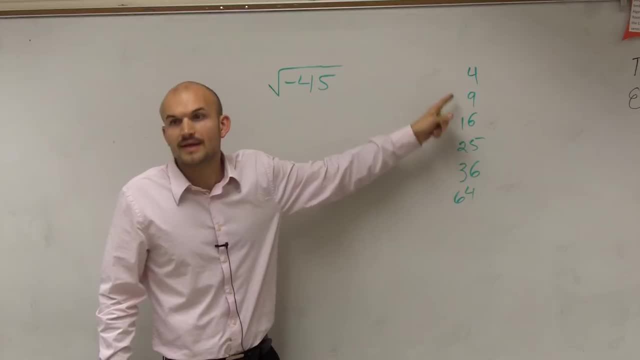 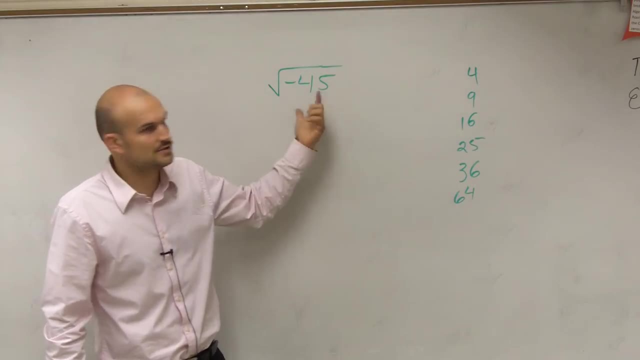 Because can we take the square root of all these numbers? Yes, So if I can get one of these numbers under my square root, I can find the value. So you're going to want to factor 45.. So you guys can factor 45 many different ways, right? 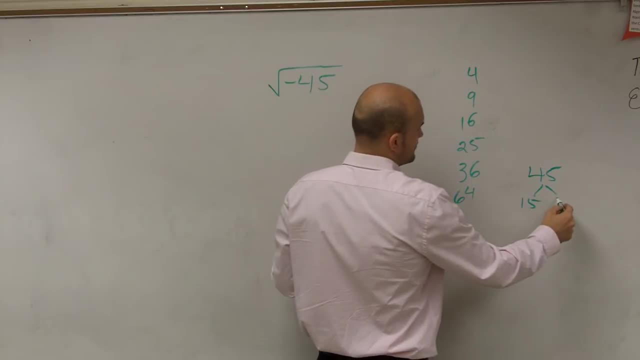 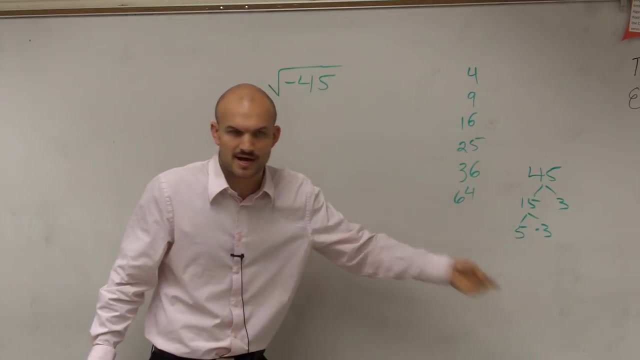 You guys can factor 45 by doing the factor tree: 15 times 3.. Um, then, 5 times 3, and so forth. right, You can use the factor tree to factor it. However, you can also just rewrite it. 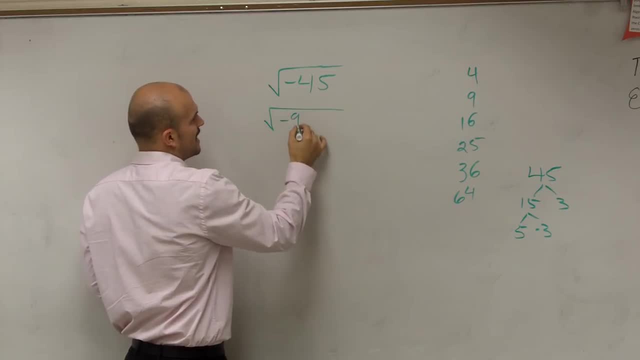 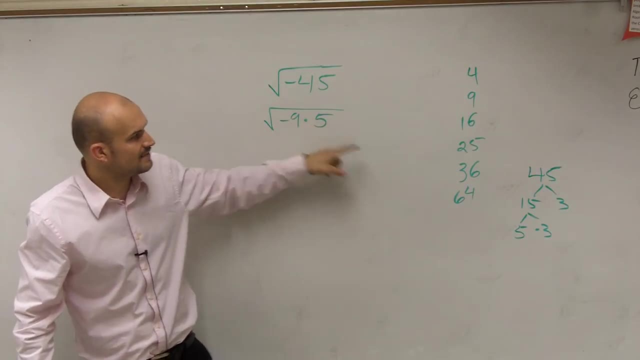 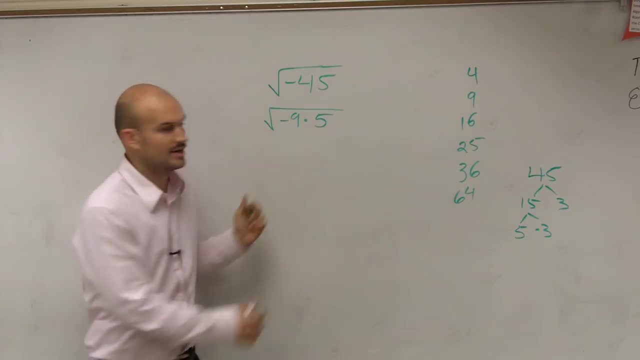 Why don't I rewrite this as negative? 9 times 5?? Is that fine? But the reason why I'm going to choose 9 times 5 is because 9 is a square number. Alright, Now I'm going to do this one more time, because I don't want a negative number there. 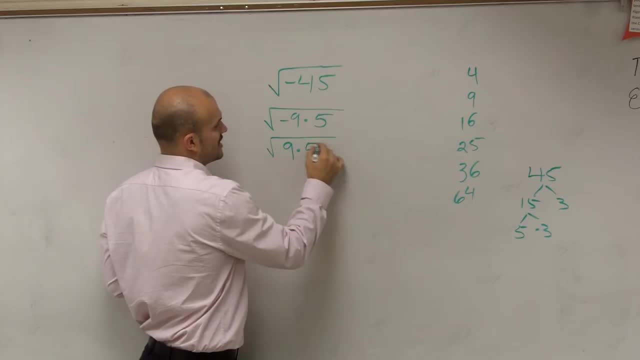 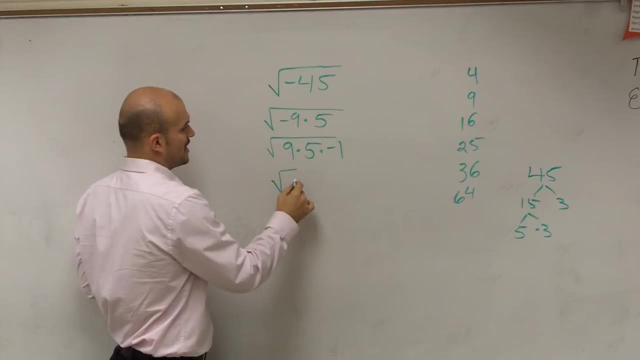 So I'm going to rewrite it one more time as positive 9 times positive, Positive 5 times negative 1.. So then, when I go and break this up, I have square root of 9 times the square root of 5 times the square root of negative 1..